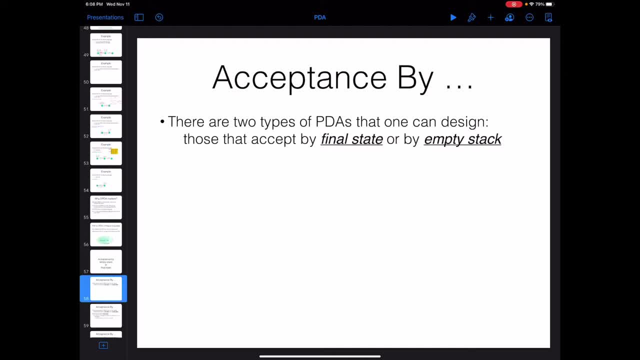 can actually design a push-down automata that accept strings by reaching to a final state state, or design or push-down automata to accept the strings by MTS stack. what does this mean? I mean, so far, all the examples that we have seen were a type of push-down automata that 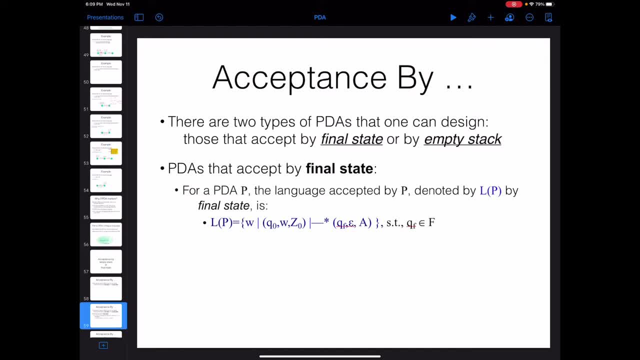 accept the strings by a final state. basically, it means that you started from the state q0 and by reading the full string w and the starting content of the stack is, the initial token of the stack is at zero. if you can reach after a couple of moves, doesn't matter how. 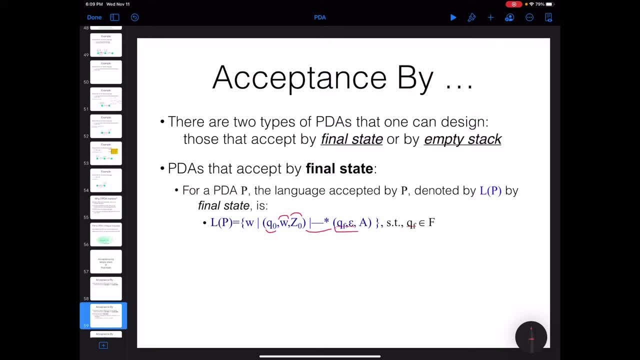 many moves. after a couple of moves. if you can reach to one of these situations that you are an accepting state and you have read the full input input string, you are going to accept the string and you can actually see that I wrote the content of the stack to be a, which means that. 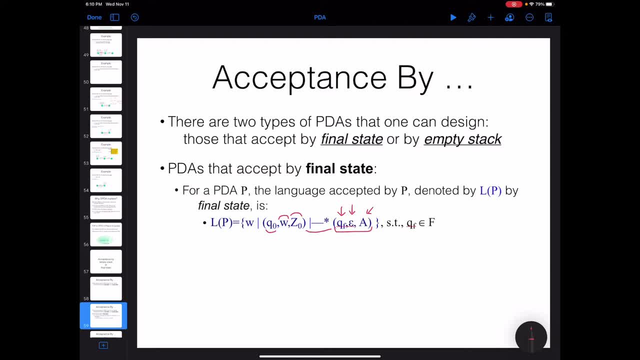 we don't really care what is in the stack. as far as we have reached to one of the final states and we have read the full input string, we would actually say that the string has been accepted. doesn't matter if the stack is empty, or basically actually doesn't matter what is in the stack. 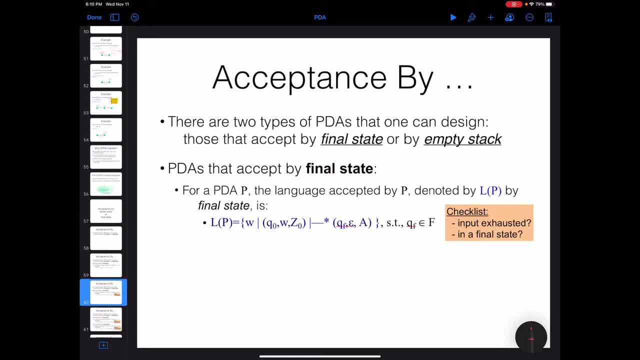 so, in this case, the checklist that you have checked out is that the input should have been consumed completely, and you should be in a final state to accept this. in addition to this specific form that we know, this is something similar to what we did for the finite state machines- that you should read the full string and you should be. 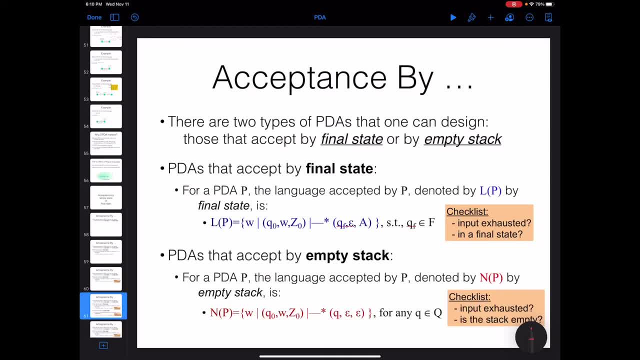 in a final state. in addition to this, we can actually design or finite or push down automata to be to accept the strings based on the content of the stack by empty stack. we call it by empty stack. so in this case, if you have designed such a pushdown automata, you would say that your 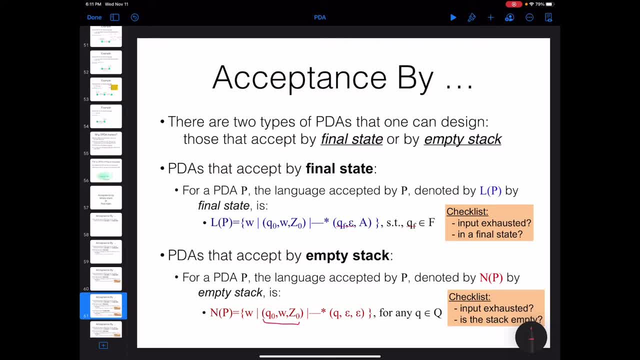 pushdown automata is going to accept all the strings like w, that if you start at the initial state, q0, and the content of the stack is z0. if you can reach, after a couple of transitions, if you can reach to a situation where you have a pushdown automata and you have a pushdown automata. 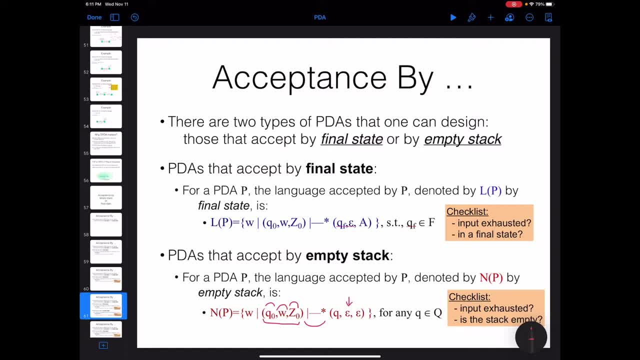 that you have read the full string. there is nothing remained in the input string and the content of the stack is empty. it doesn't matter which state you are in. you would say that you accept that string. so all of those strings w that you can start with the initial state and the. 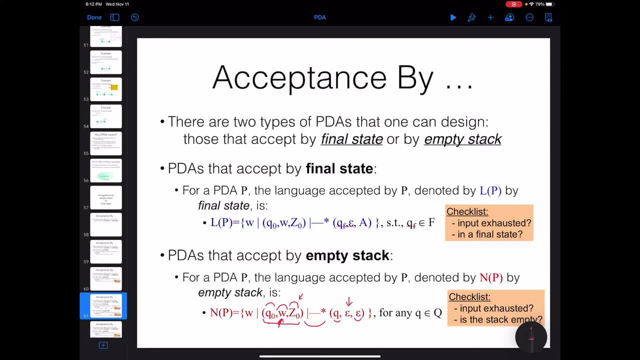 content of the stack, only the initial token of the stack: z0. if you can reach to a situation that you have read the full string and there is nothing in the stack, everything has been removed from the stack, including z0. in that case you would say you accept this thing and it doesn't matter which. 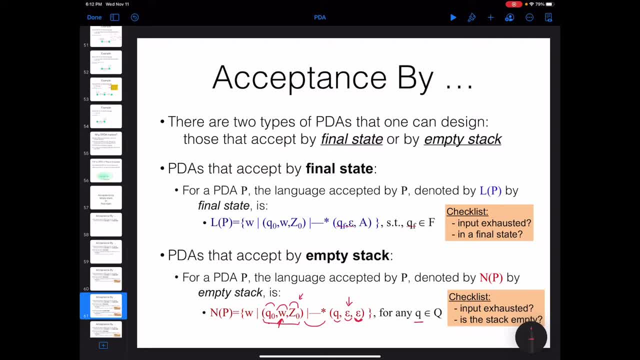 state you are in. okay, so this type of pushdown automata doesn't really care about the state of. we don't really need the final state. not only we don't need a final state in this type of pushdown automata, but we can actually see that we don't need different type of states as well. only one state is going to be enough if you design your pushdown automata to accept the string by empty stack. 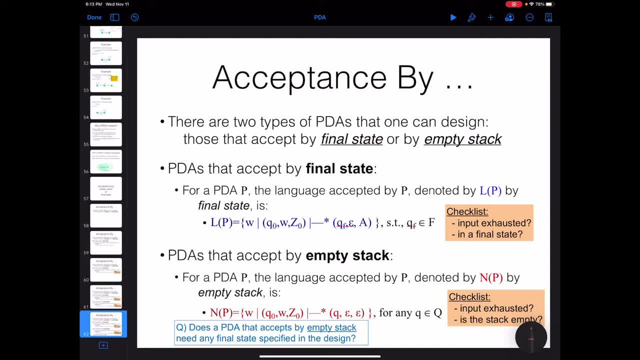 you know, basically the pushdown automata that accept by final state are going to be more. you know, when you are designing your pushdown automata, it actually makes it much easier if you design it based on final state. it's just like you write down some algorithm and 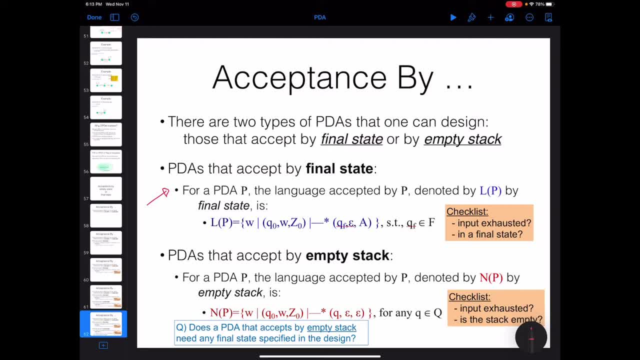 you just follow that. just okay in this state, just push in this state, just, for example, pop and then go to the final state in an accepting state, and then you can just have a final state. but the empty stack pushdown automata basically actually tells you that when 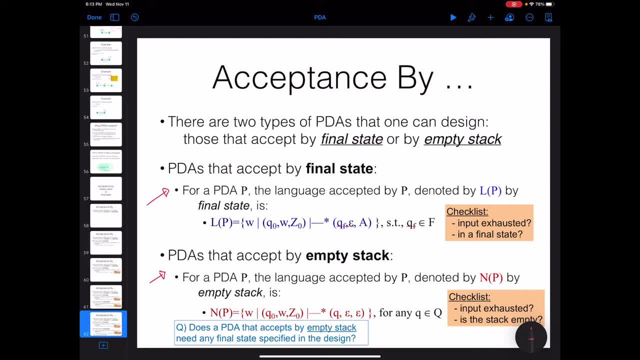 you are designing a pushdown automata, your finite state doesn't need to have different type of states. we just care about the actions that you do over the stack. we just make sure that. we just wanted to make sure that you read the input stack and after a set of actions over the stack, stack is empty. 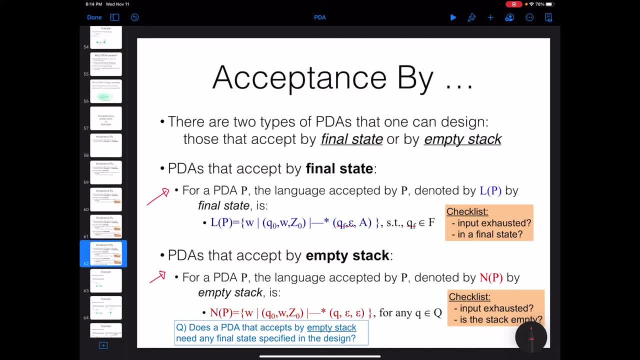 um, so we will see that these two type of pushdown automata- it doesn't really matter that if you have designed your pushdown automata to accept by final state or you design it to accept by empty stack, and these two types are going to have the same power. i'm going to show you that they are. 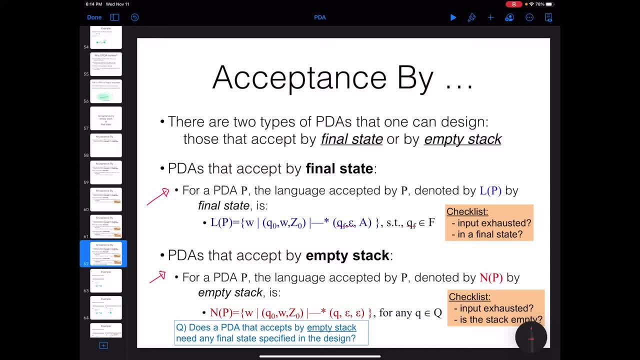 equivalent. it means that if you have designed a pushdown automata that accept by final state, you can convert it to a pushdown automata and you can see that it's going to have the same power that i accept by empty stack and vice versa. so before i'm actually proving the equivalency of 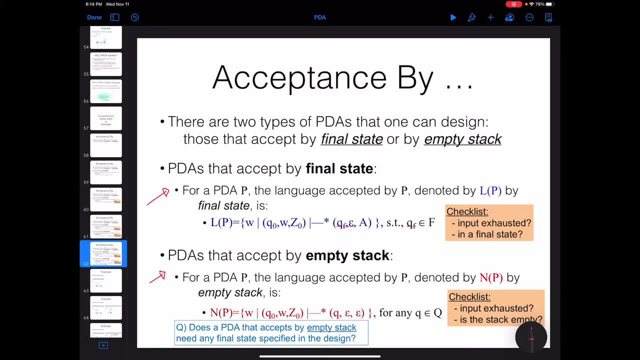 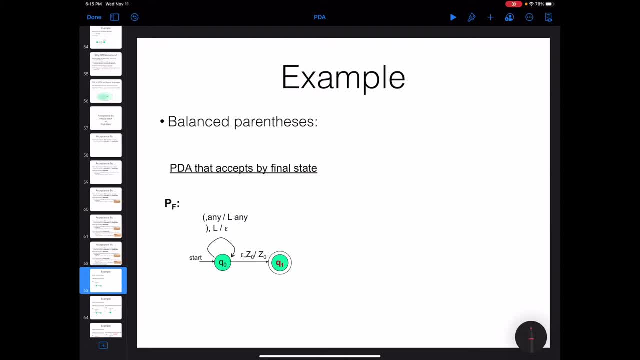 this type of pushdown automata, these two different pushdown automata. i'm going to show you an example. assume that we are working on the language of balanced parentheses, so basically, the sigma, the alphabet, is going to be just the two tokens, the uh, closing and opening parentheses. right, and we wanted to um design a pushdown automata. 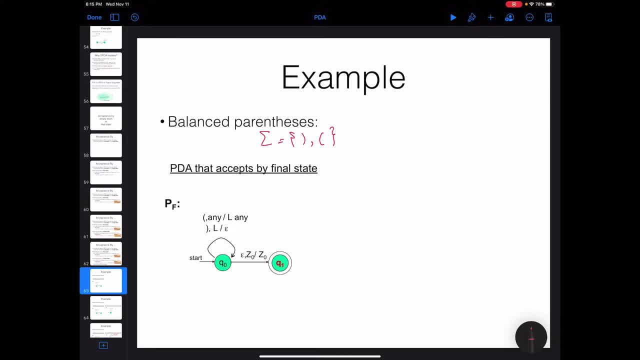 by final state that accept all the esterings which are balanced in terms of the parentheses. so this is going to be a pushdown automata, that except for final state. okay, so you can see that basically, in the state q, zero for every open parentheses that we will see doesn't matter what is the top of the stack. 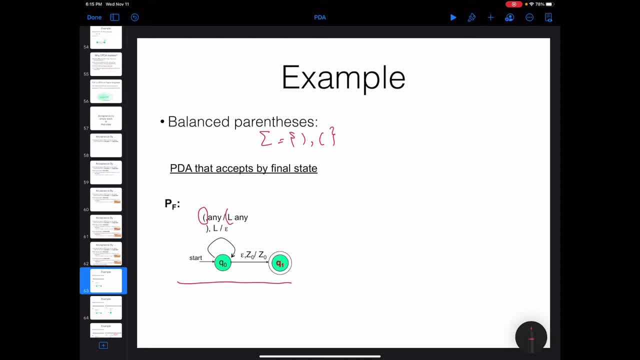 just actually push, you know, a token to the top of the stack, and for every closing parentheses the top of the stack should be an opening matching to that and you pop it and you basically only go to the accepting state whenever you have read the full string and there is no. 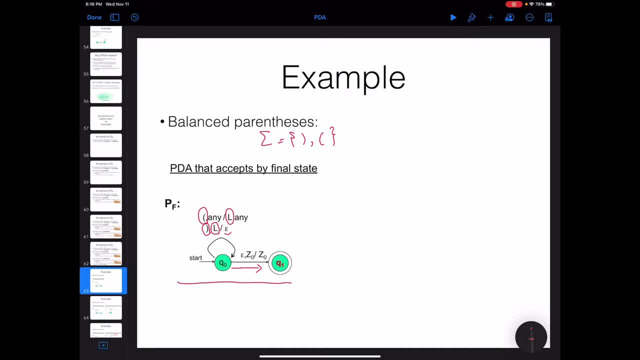 token, except the z0 in the top of the, on top of the stack, and you go to the final state and you would accept it. it's actually um, it's very- um, you know, intuitive. now i'm going to show you an equivalent pushdown automata that accept the same language. 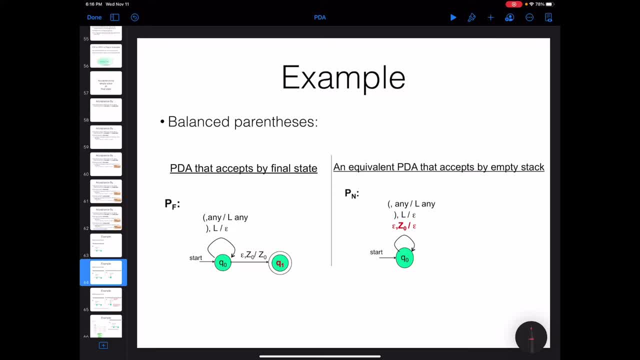 um by mts stack. uh, it doesn't have a final state. we actually don't need a final state, um. so, basically, this pushdown automata is going to be very similar to this one, the only thing is that we don't need the accepting state, and i'm going to add one more: transition over q0. 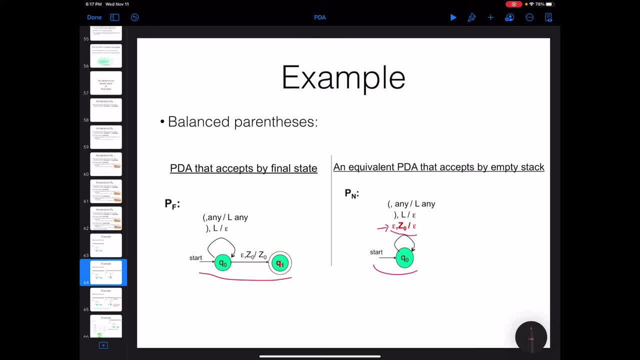 and that transition. basically just remove the remove the z0 from the stack, um. so when you are actually doing such a um you know action, it means that, without consuming anything from the input string, if you remove z0, um, it means that there is nothing in the stack and if z, even z0, has been removed from the stack, you cannot do any other action. 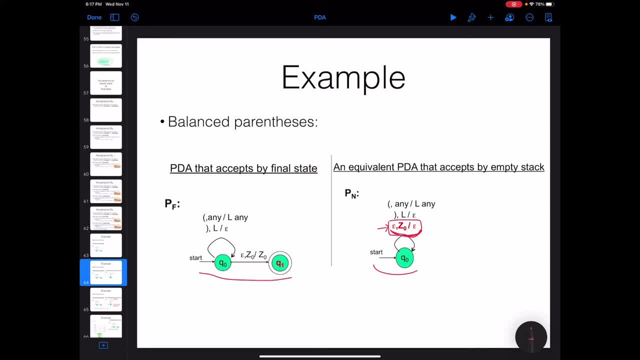 so in all the pushdown automata you can do any other action. so in all the pushdown automata you can do any other action. so in all the pushdown automata you can do any other action. so in all the pushdown automata that you design based on. 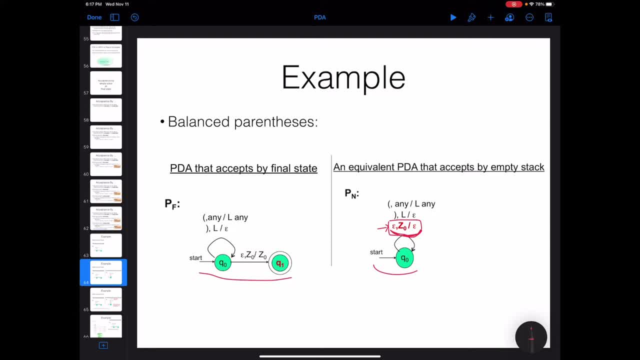 empty stack. you should remove z0 because the stack should be empty at the end. okay, and it is important that you actually note that after removing z0, it basically means that we cannot do anything else. none of the. there is no transition after you have removed the. 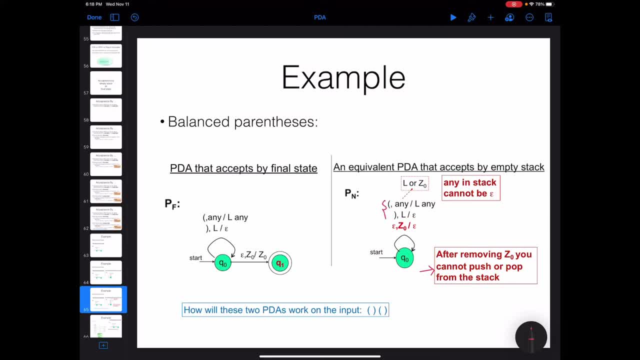 z zero, because none of this transition can be done and you are done if you remove the z zero. it's just like this is the, the end of the, the program you are. you can't do anything else. to make it more clear how they works, how these two different machine works, i'm going to show you how. 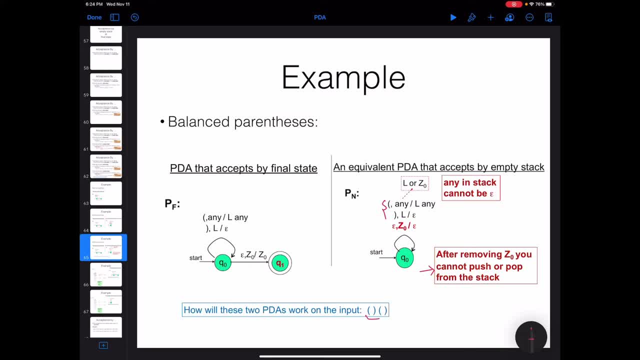 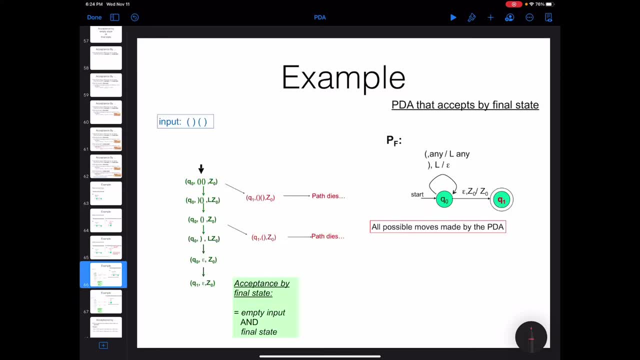 they works on this input string which is in the language. this is a valid string. okay, the first one is the pda that i accept by final state. here i'm actually showing that how the machine is going to work and check all the possible moves for this input testing and clearly this is not a deterministic. 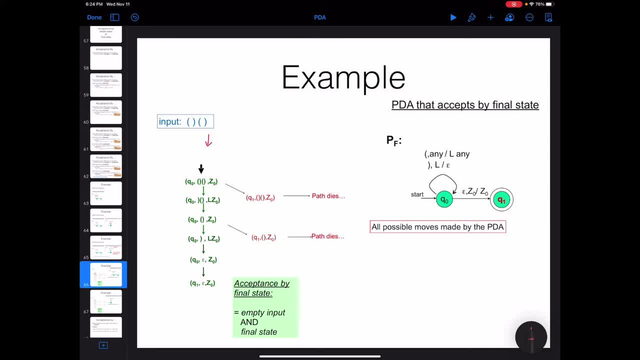 pushback down automata. this is a non-deterministic one. you can see that at the beginning we will start at this situation: that we are at state q0, the full string hasn't been read yet and the token on top of the stack, the only token in the stack, is the initial token, z0. 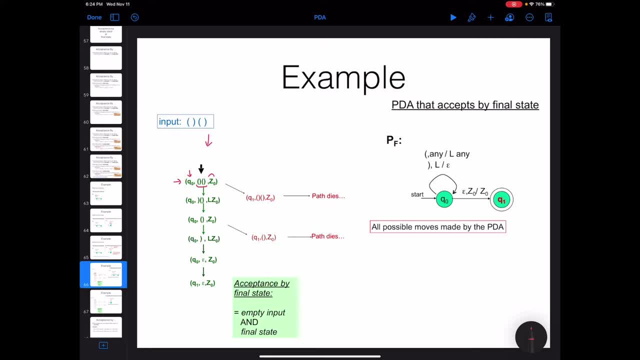 so at this situation, there are two possible moves. you can, either, because the top of the stack is zero, you can either move to q1- right, we don't actually can see that at this point, so you can actually reach to this configuration- or you can use these transitions that tells you that it doesn't matter what is on top of the stack if it is z0. 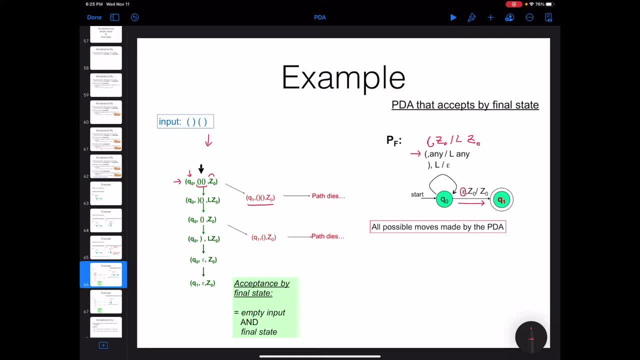 or, if it is l, you can stay at q0 and push and a token l to the stack. okay, so there are two moves. clearly, this move is going to crash because if, after you move to q1, there is no more action, there is no more transition for q1 and you haven't. 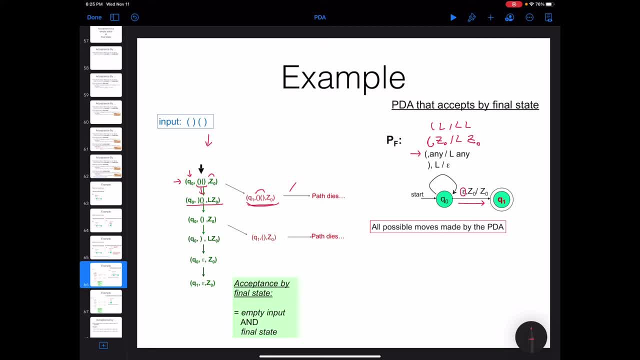 finished the input string, so this path is going to crash and this is not going to accept, and you have to continue this state. at this state, there is only one possible transition for us. you are at q0 and the top of a stack is l, so the only thing that you can do is that. 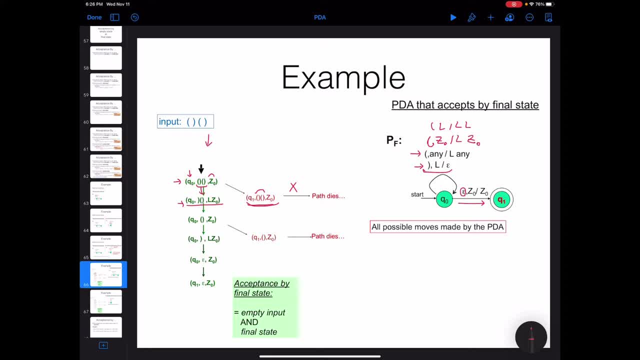 you are at q0. the top of the stack is l and your input strings are that. your input string is the next input string is a closing parenthesis, so you have to match it to the top of the stack. you remove the l from the stack and they stay at q0. so there is only one possible move for you. 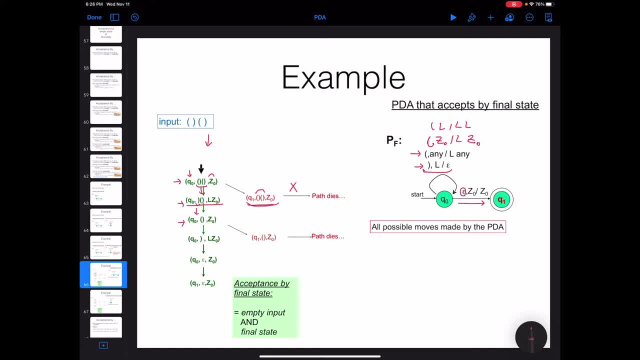 here at this situation again. you can see that there is nothing in the stack except z0. the top of the stack is z0, which means that you can use this transition and go to q1 without reading anything from the input, and it is clear that this is going to die again you, this is going. 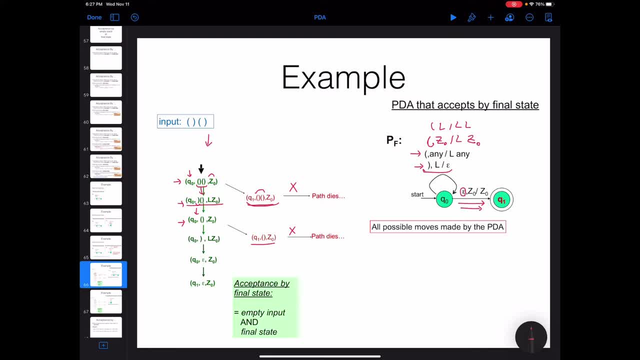 to crash because there is no transition at q1- um and you haven't read the full string yet. the other action is that you can push a token l to the top of the stack by reading the open parenthesis from the input and stay at q0 again. at this situation, there is only 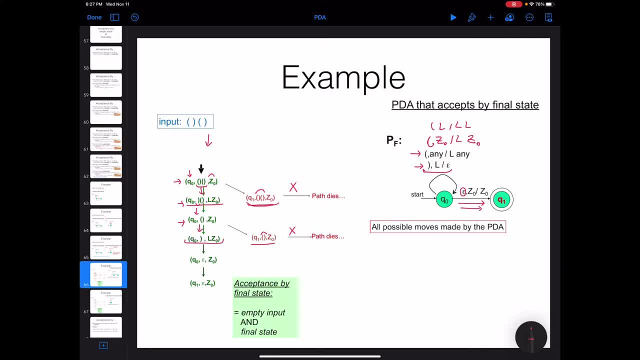 one possible transition: the. you are at q0. the next token is closing parenthesis. the top of the stack is l, so you remove l from the stack, which means that you have matched a token, an open parenthesis간, which means that you have matched a tokenpan and open, so the token is open and you can't go into this transition. if the. the stack is closed continuous. prefer to go to q2. 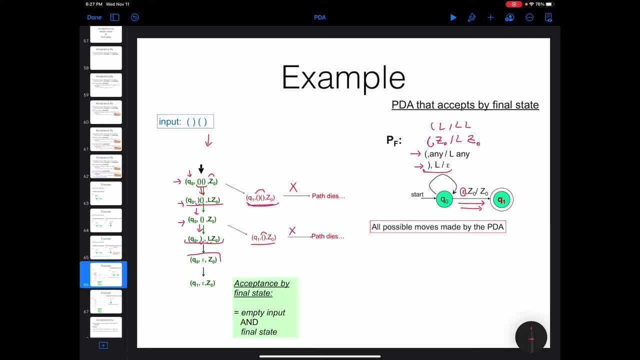 open parenthesis with this closing parenthesis and you reach to this situation and at this situation, the only transition that we have is because we have read the whole input string, so we can only move to state q1. we have finished the input string and, yeah, we are going to accept the string. so this: 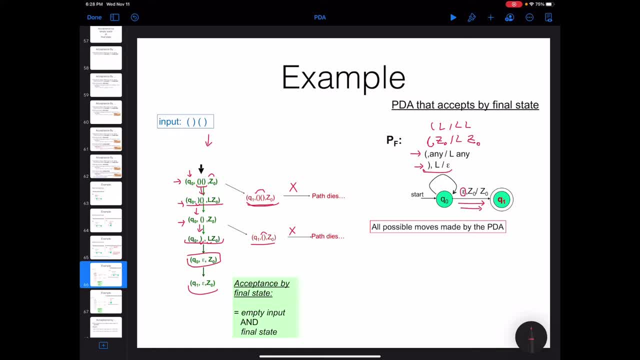 is the way that we work on a pushdown automata that accepts by final state. you have to reach to a final state and you have to finish the input string. now i'm going to show you that how the other pushdown automata that accepts by mts stack is going to work. at the beginning, you start at q0. 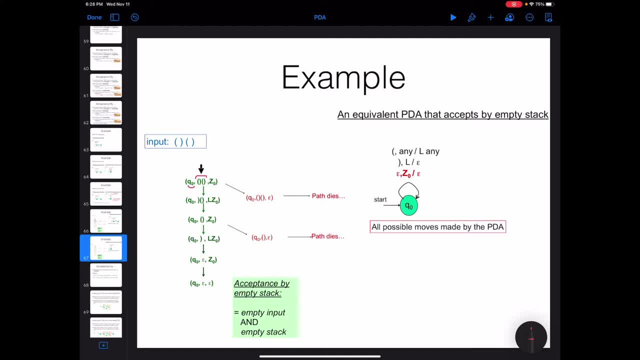 the full input string hasn't been read, we haven't actually started yet- and the top of the stack is zero. based on the transitions that we have here, you have two transitions right. you can either use this transition to remove- um, i mean without reading anything from the input string- just remove the z zero from the top of the stack. 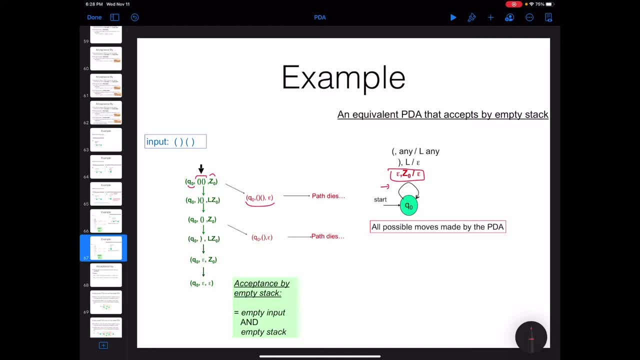 and reach to this situation. um, so this path is going to die again, and the reason is that, um, this part is good, that we don't have anything in this, like a stack is empty, that's good, but we haven't read anything from the input, so you are not done. and you i mean basically the machine. 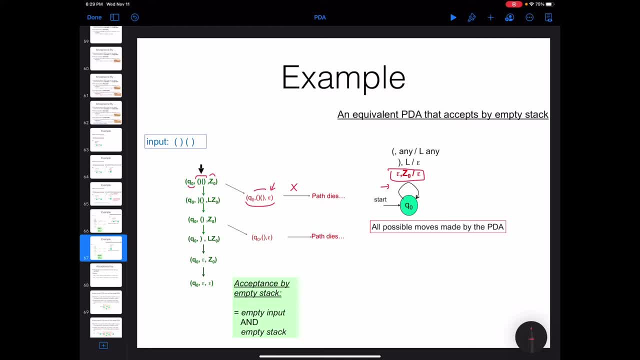 will crash and just reject this right. the other um possible action is to use this. as to this transition here: um, we use the consume- one input string and then use the same action on the other string. one token, the first token, which is an open parenthesis, push an l to the top of the stack and 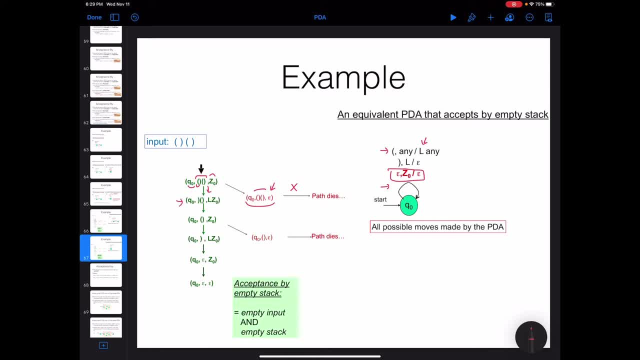 reach to a situation like this, at this position, there is only one possible action, which is this transition which tells you that you are at the state q0. you stay at q0, you read this input steering and you pop um one token from the stack. so you reach to this situation again here, there. 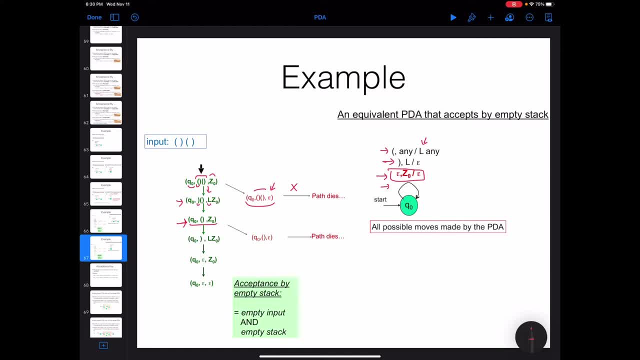 are two possible transitions. you can either use this transition and remove z0 and you can see that after removing that zero, you can't do anything else and you haven't finished reading the full string. so the this path is going to be: it will die. so you can't actually accept the string. 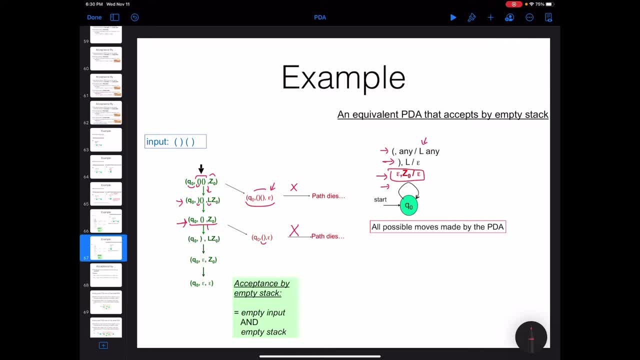 in this path. you have to be able to do all the operations like this. you have a lot of time you to continue with the other transition from here. that's actually using this transition that push another l to the top of the stack. use the first, actually consume and read the first. 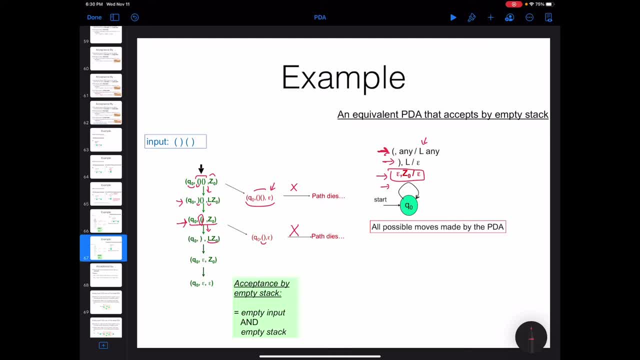 the next token in the input string and push an l to the top of the stack. and here there is only one possible transition, that is, popping and l from the stack, reading the next closing and popping an l token from the top of the stack. and this situation- there is only one possible transition. and 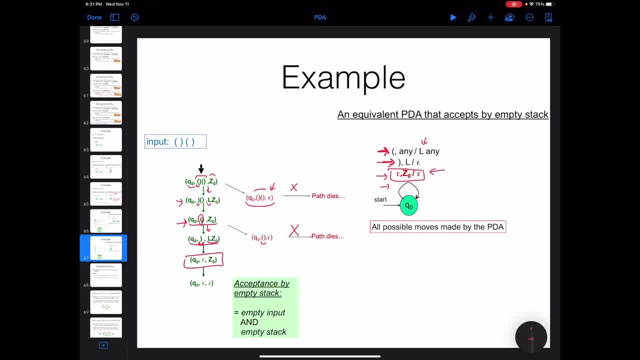 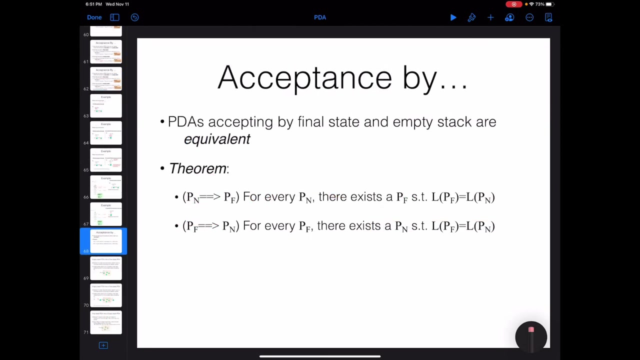 this is the transition that, basically, is going to be the final transition. it just makes it remove the last token from the top of the stack, which is the zero, and you reach to this situation, which is an accepting situation. you have read the full input string and the content of the stack is empty, so you would accept the string. so i'm going to now. 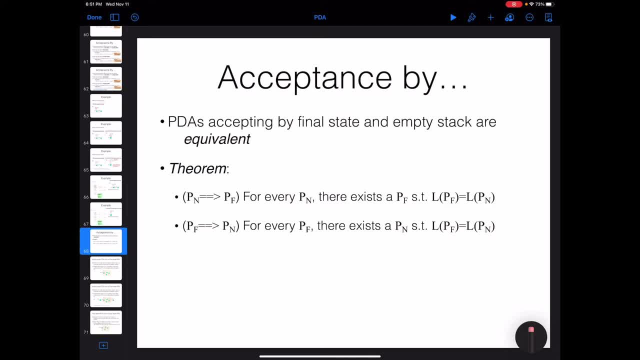 show you that um, it doesn't matter if you design your pushdown automotive by um, i mean accepting by final state or empty stack. they are equivalent, they don't give you more expressive power. so i'm going to show you that if you have a pushdown automatic, that except by mts stack. 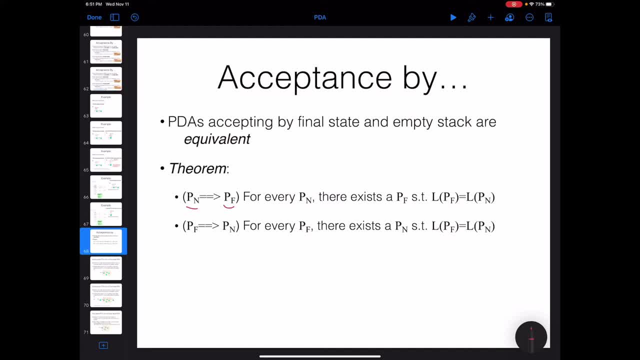 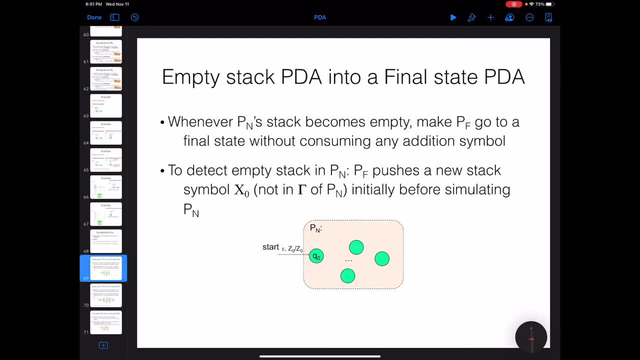 you can convert it to a pushdown automata that accepts by final estate and vice versa. so these proofs are again constructive proof. um, so just assume that if you have a pushdown formative that I accept by empty stack, I am going to how to convert it to a push non-automata that I accept. 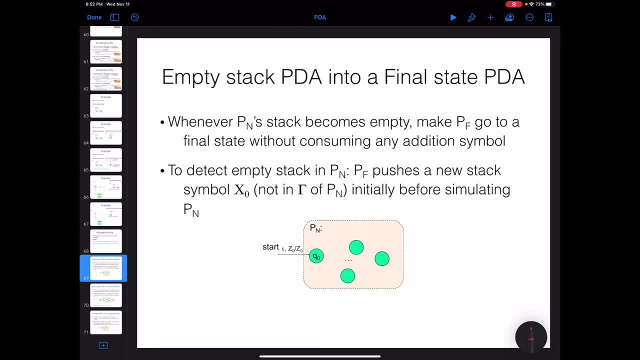 by final state. I'm going to add a new token. be careful, this token shouldn't be in the alphabet of the stack. I'm going to add a new token and consider it as the initial token of the stack in the new push non-automata that I'm going to create. okay, so this is going to be a new. 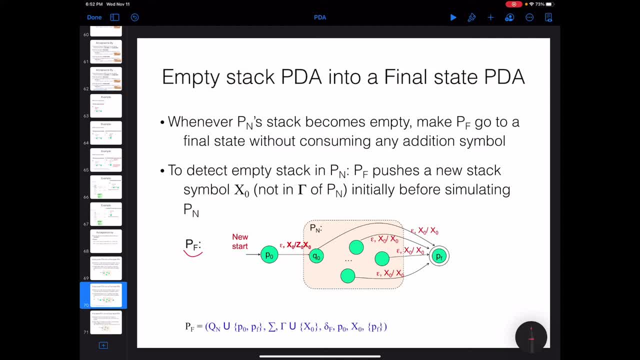 push non-automata. x0 is going to be a new token that I'm going to consider as the initial token of the stack. I will add a new state, a new initial state and just from this initial state move to the initial state of the the. 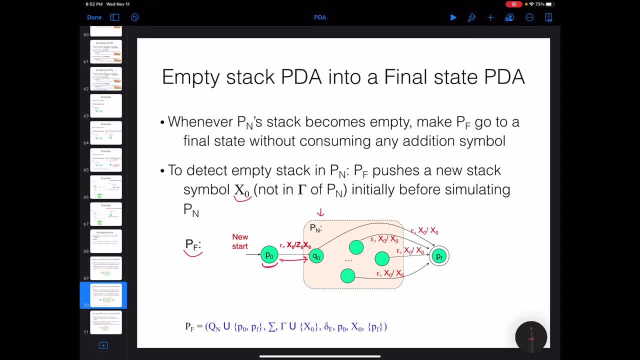 original push non-automata and the action is: you don't actually consume anything from the input, we just push, in fact, x0. just make sure that x0 is in the stack and over this transition, z0 will be pushed on top of x0. okay, so now when you reach to any of those situation, 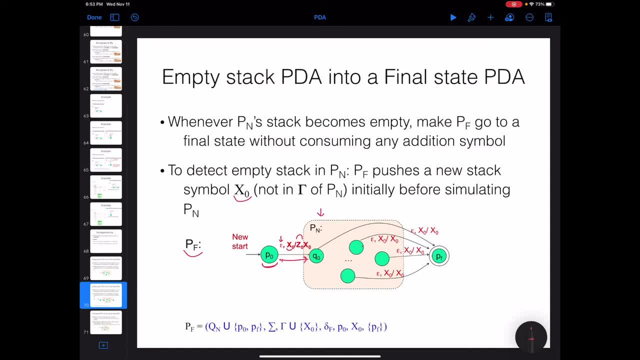 that do that. you, um, you are going to accept the sring and in those situation you remove z0. it means that you are at a situation and you remove zero, you don't have z0, right. you are accepting your push down automata by MTS stack. 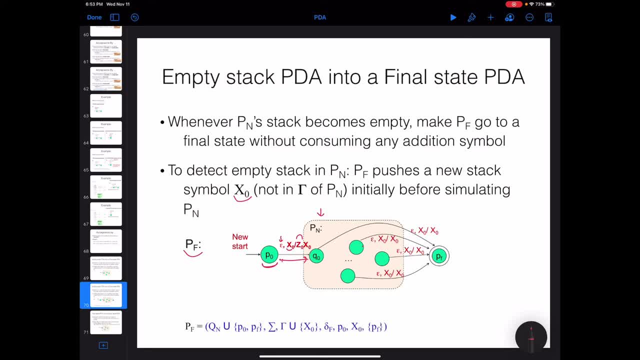 but no, in all of those cases you are going to have x0 there, right? because x0 is there before, Or even Z0 has been pushed in this new push-down automata. What I'm going is that from all of the states in your original push-down automata. 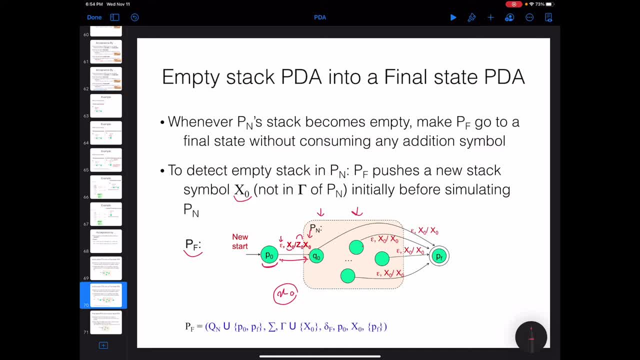 I'm going to add a transition to a new final. I said the final state is going to be unique From all the states in the push-down automata, because you can actually accept a string in any of these states, right? The requirement for accepting is that the stack should be empty. 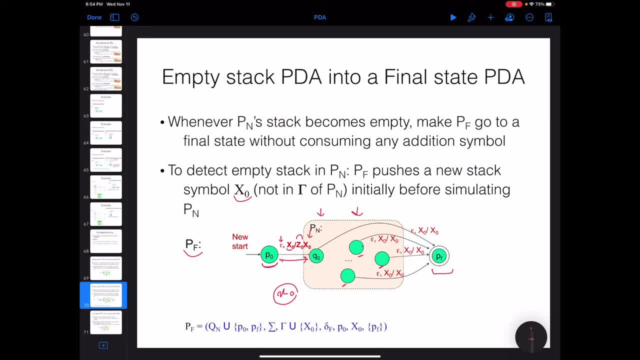 From all of these states, add a transition to an accepting state And that transition basically just doesn't actually consume anything from the input. so epsilon from the input, But it actually forces you to have X0 as top of the stack, which means that it's just like in your original push-down automata. 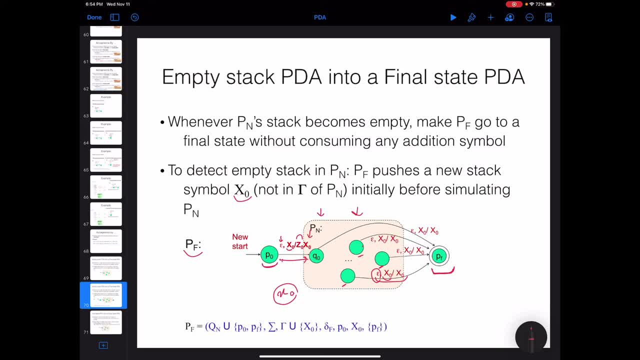 the stack is empty. Even Z0 has been removed, right? In that case, just move to the final state. So we are going to add a transition over all the states, but this transition only moves to the final state if the top of the stack is X0, right? 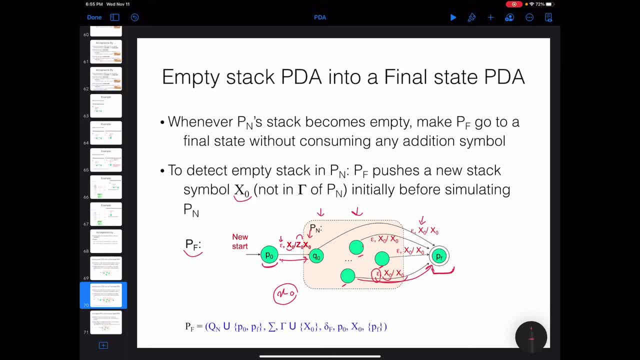 And so this new push-down automata that has been created is going to accept exactly the same language. All the strings that will be rejected will be rejected in this new, and all the strings that will be accepted will be accepted in this new push-down automata. 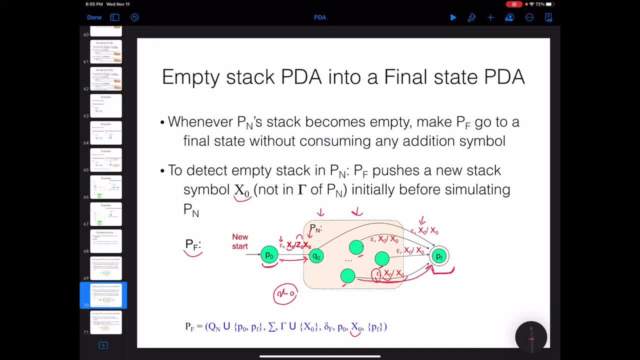 And you will see that. just make sure that the new initial state, the new initial token of the stack is going to be X0, not Z0 anymore, And we have a final state which is just whatever you call it: P, sub F. 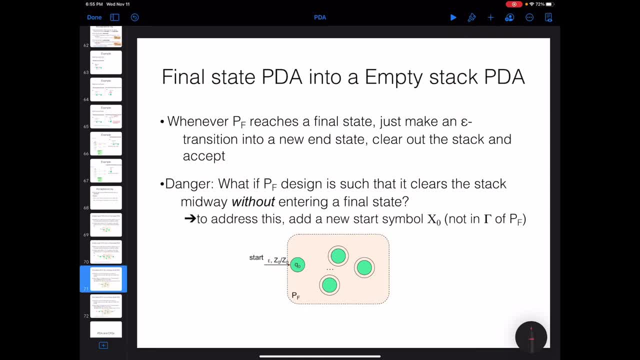 So the other part of the proof is that I should show you how we can convert a push-down automata that I accept by final state to a push-down automata that I accept by empty stack. So just assume that I have a push-down automata that I accept by final state, right? 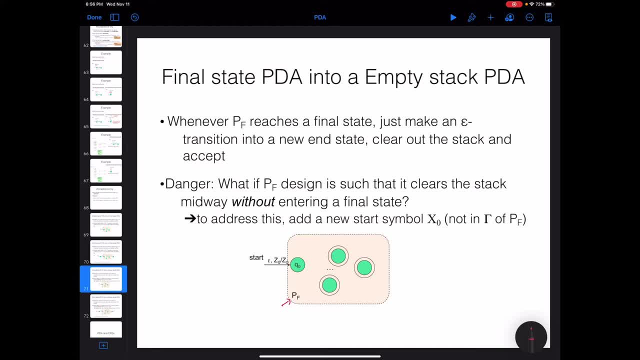 I can have as many number of final state as I want. It doesn't really matter how many, But to convert it to a push-down automata that I accept by empty stack, the only thing that I need to do is that. just make sure it doesn't matter from which state you are. 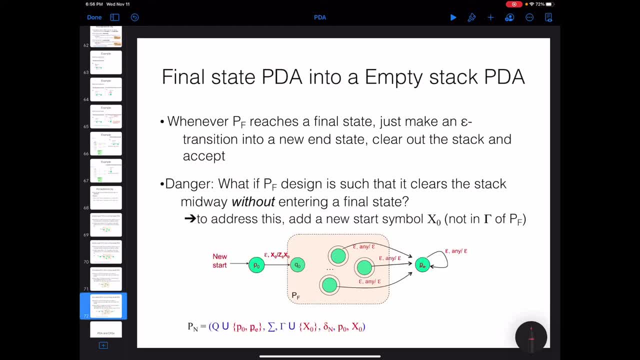 just add a new in all of these final states. in fact, the thing is, you don't know what is in the stack and you don't care what is in the stack. You only care that you reach to those final state. 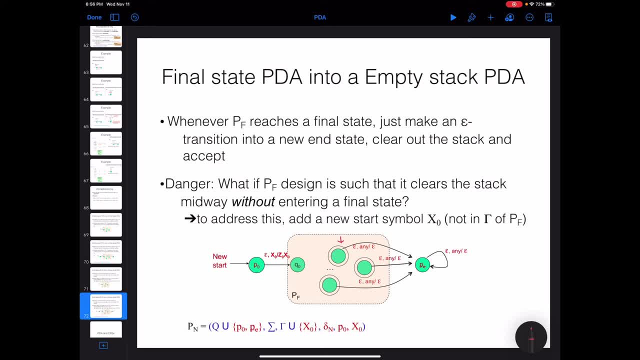 and the input string has been consumed totally. So you would accept the string. But to convert this final state, this push-down automata, to a push-down automata that I accept by empty stack, the only thing that I need to do is to just empty the stack at the final states. 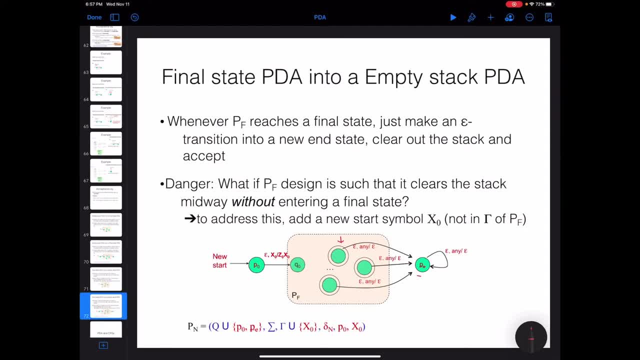 So I'm going to just add a new state, okay, And move from all of the final states, add a transition from all of the final states to this new state. You see that we don't consume anything From the input, it's just you're moving over epsilon. 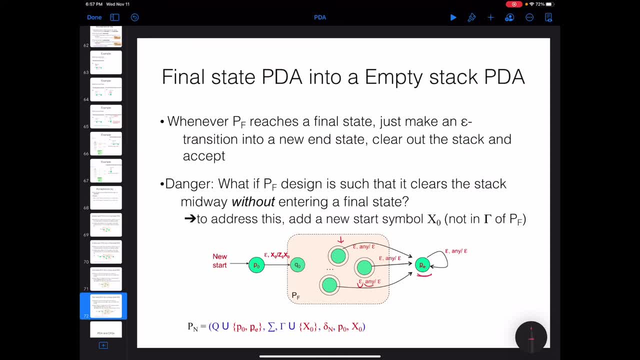 and we don't care what is the top of the stack. Whatever it is, the top of the stack does, just remove it. Okay, whatever is the top of the stack, just remove it. Whatever is the top of the stack, just remove it. 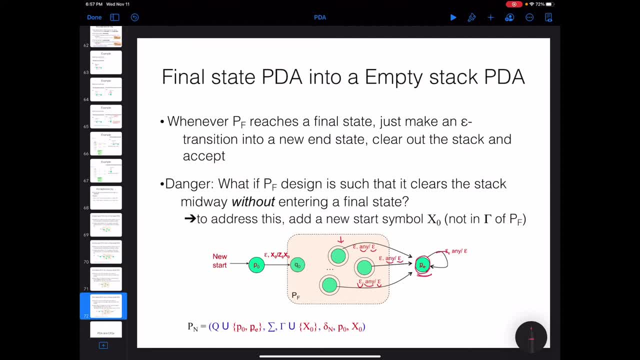 And in this state just keep removing all of the tokens in the stack. So we don't actually putting any constraint over the string or anything. We just remove all the content of the stack, So all the strings that has been accepted by the previous push-down automata. 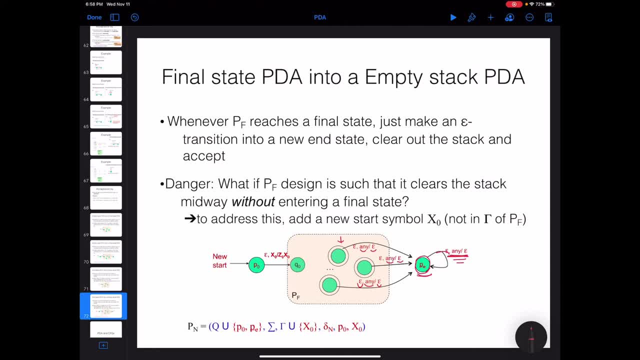 they are going to be accepted here as well, because we have a transition to remove all of the content of the stack Here. just one thing that I have showed to add x0 here as well, but it doesn't really matter. You don't really need this x0 to add for this case. 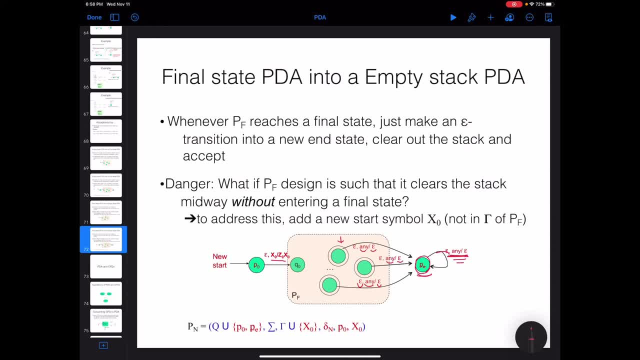 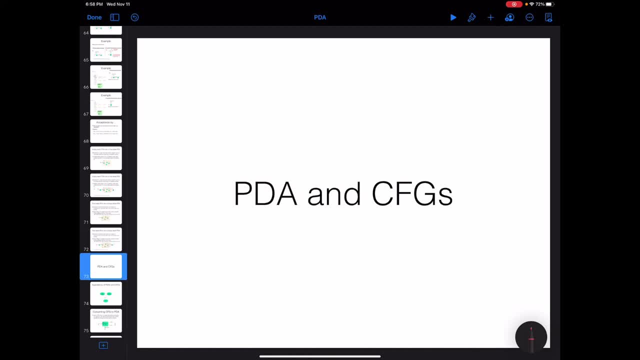 But I just wanted to actually keep it formal, Okay. the next topic to discuss is the equivalency of push-down automata and context-free grammars. Basically, we have already talked about the context-free languages and context-free grammars, that any language which is context-free. 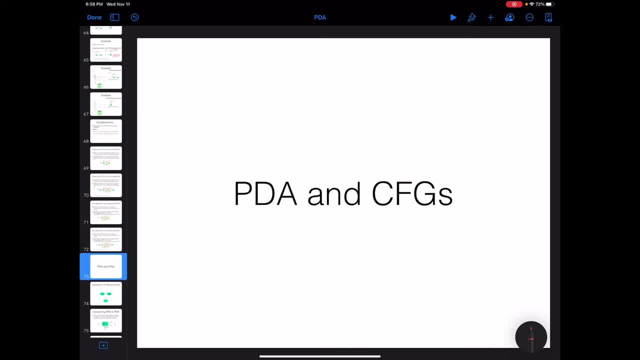 we should be able to create a context-free grammar for that, And the push-down automata is a machine, is the type of machine that accept the context-free languages. So we should prove it. We should prove that if you have a context-free language, 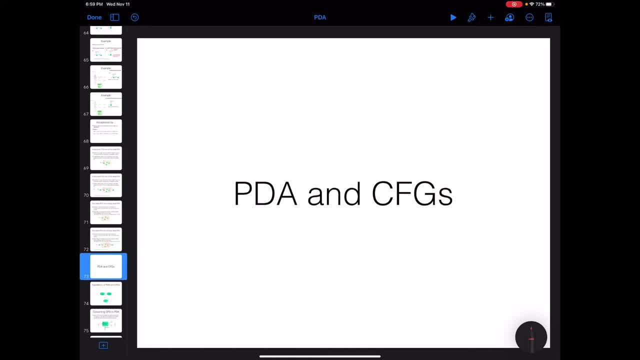 you have to accept it. So we should prove it. We should prove that if you have a context-free language, context-free grammar, you can convert it to, you can create a push-down automata that accept exactly the same language and if you have a push-down automata, you should be able to create a context-free 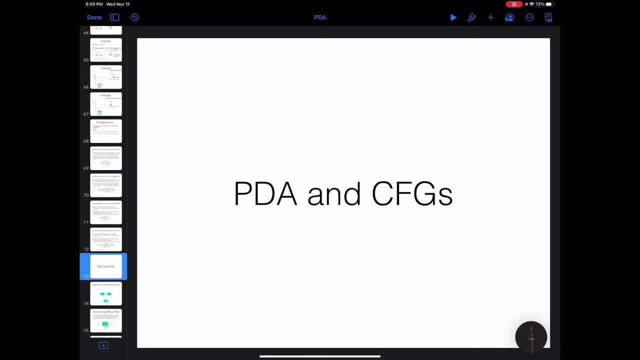 grammar that accepts exactly the same language. so in this- actually a slide- you can see that we already actually know that. the push: it doesn't matter if you have a push-down automata that accept by final state or empty stack. they are equivalent. we can convert them to each other. 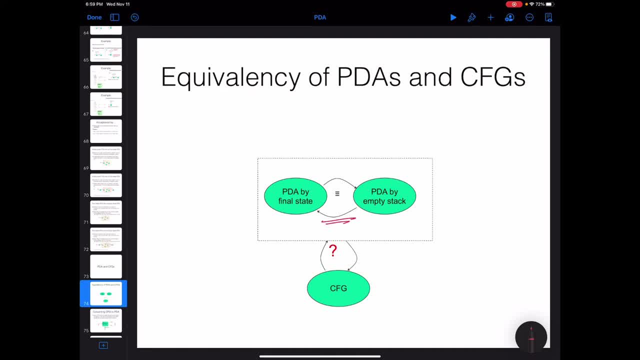 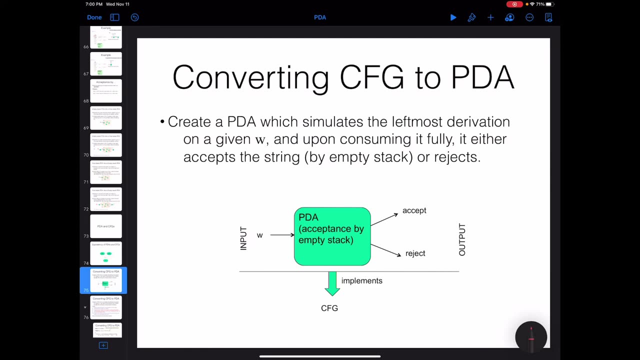 and now i'm going to actually show the relationship between them and the context-free grammars, basically how we can approve they are equivalent. so first i'm going to show you how to convert if you have a context-free grammar, how we can create an equivalent push-down automata. 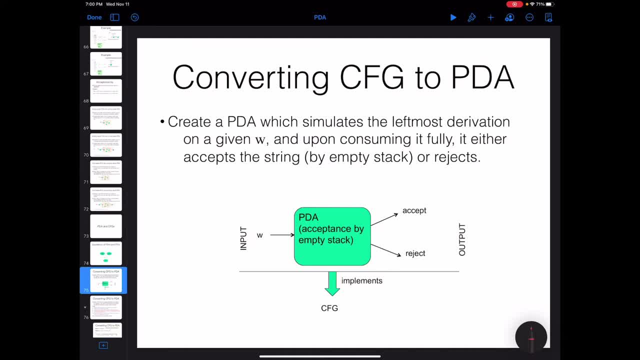 for that and that is going to be a push-down automata that accept by empty stack. basically, the reason that i have discussed about this- i mean the push-down automata that accept by empty stack- is that all the proofs that we do over the context-free languages and 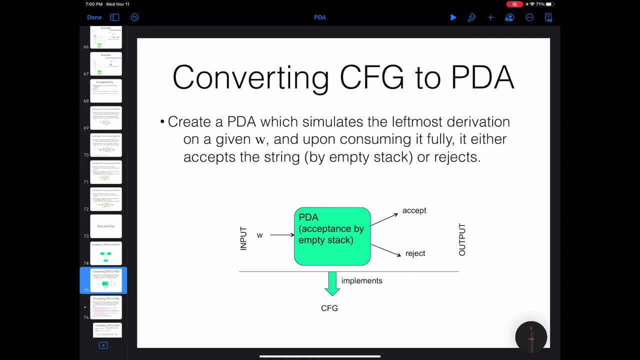 push-down automata are basically working on the push-down automata that accept by empty stacks. so this is just like a more theoretical representation for the push-down automata. so this, um, this part of the proof that, proving that any for any context-free grammar we can create. 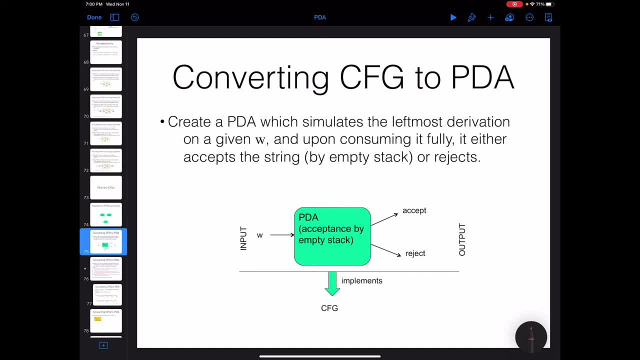 a push-down automata. this is a constructive proof. i'm going to show you that, if you have a context-free grammar, how we can create an equivalent push-down automata that accept the same language. so basically all the, which means that all the strings that i will be accepted by a 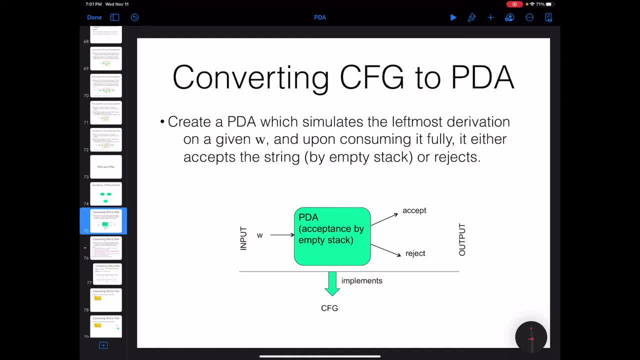 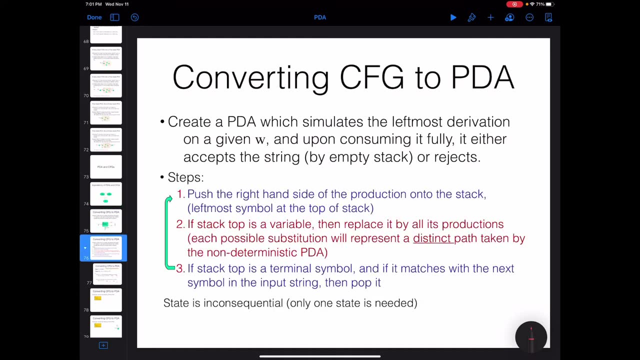 builds that will be generated by the grammar, they will be accepted by this push on automata, and if, uh, there is any thing that will be rejected by this push-down automata cannot be generated by the grammar. um so, um, these steps that i've written here, 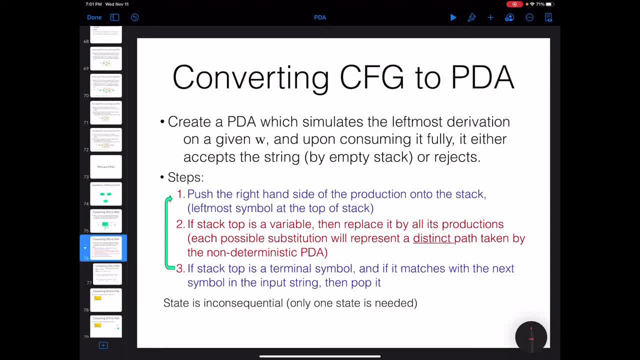 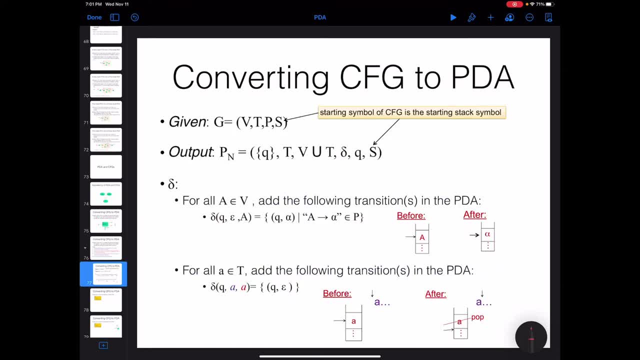 is just a verbal explanation of that. i'm going to skip this slide and basically just show it to to you over an example. But before explaining the example I am going to actually just briefly discuss that: what type of transitions we are going to have in this push down automata. 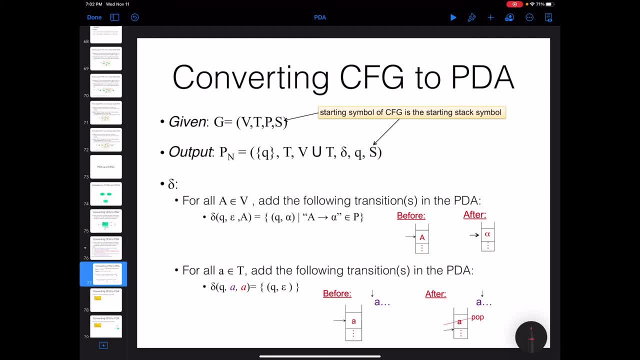 We have a context, free grammar. we are going to create an equivalent push down automata for that which this push down automata is going to accept by empty stack, and we are going to have only one state in this push down automata. Okay, so we don't care about the, the states, the only. 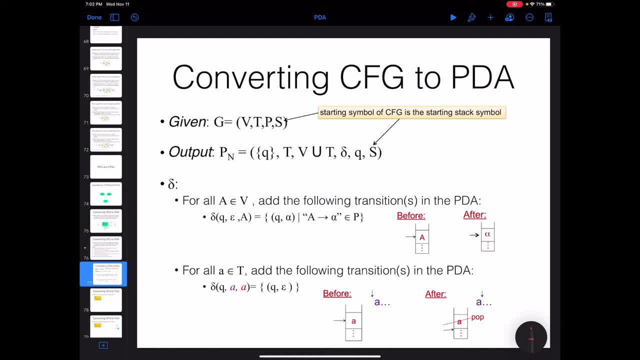 thing that we care is that is the transition. We are going to create all the transition in our push down automata using the, the rules that we have in our grammar. So what we have as the input is the input of the grammar. So what we have as the input is the input of the grammar. 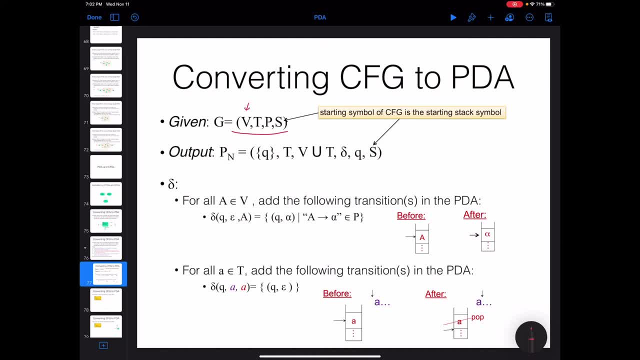 So what we have as the input is the grammar, which has a set of variables, a set of terminals- remember- a set of rules and the initial, the starting symbol in our grammar, which was the one of the variables right, we usually call it s We are going to create and a push down automata. 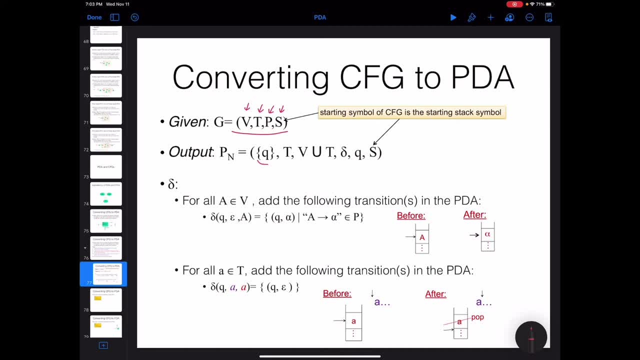 that accept by empty stack. we are going to have only one state. basically, one state is going to be enough. we don't need a multiple. We are going to have a set of variables and a set of rules and enough. we don't need more than that. and the input alphabet is going to be all the terminals. 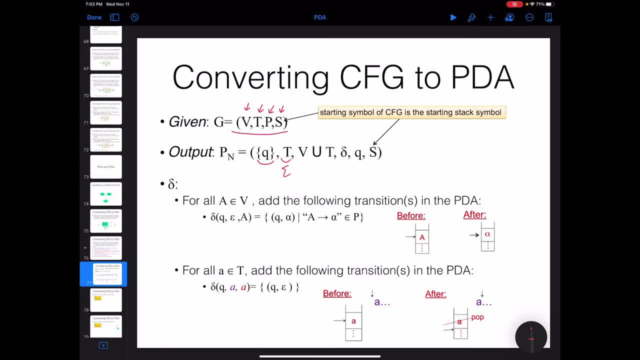 right. this is actually telling me that what is the sigma in my pushdown automata? all the terminals in the grammar is going to be the alphabet right. the variables are going to be sorry. the tokens that can be pushed to the stack are going to be the union of the all the variables in the grammar. 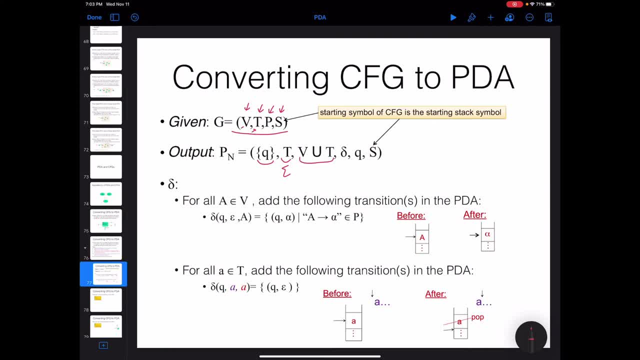 and all the, the terminal symbols, so you can push not only variables but also the, the input, the- sorry- the input alphabet into the stack. we are going to define this transition function and whatever, whatever, what else we have we don't have actually an accepting asset. this pushdown automata is going. 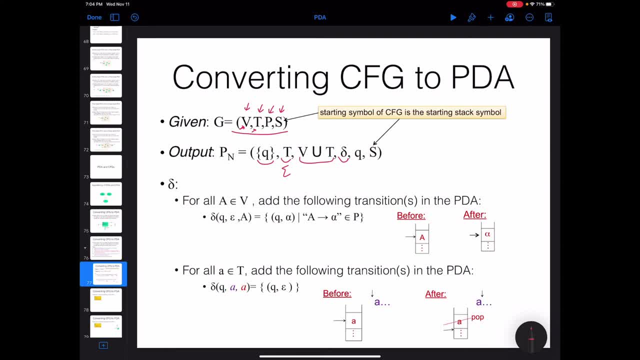 to accept by empty stack, and the initial token of the stack is going to be s. okay, note that s was the starting symbol in our grammar as well. here it actually tells you that the initial symbol of the stack- what we actually have in this, like at the very beginning- is going to be the same starting symbol that we have for the. 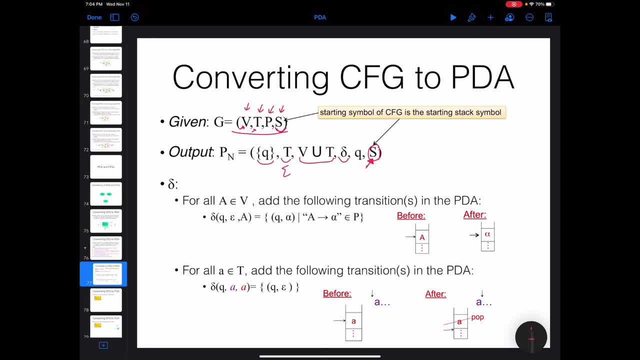 grammar. all the transition that we need to add can be defined, can be divided, actually, to two types of transition. i'm going to first explain this one. basically, these transitions are about the terminal symbols. it tells me that if the input, um, if you are at a stage where you are at a stage where you are, 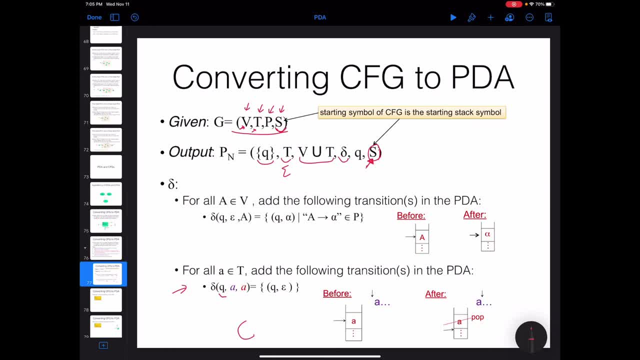 at Step, you are at the start, q 2. if you are at a state q, we only have one, a set, to be honest. okay, you are at the state q if the input string, if the input token, the next input token, is a, which is a terminal symbol, which is one of the input alphabet, right input alphabet, the Sigma, and if the top of 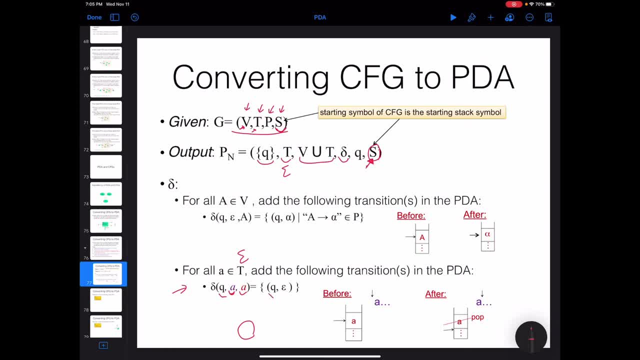 top of the stack. the transition is that you just- um, you actually read this token from the input string and you remove that token from the stack. okay, so this is for all of the tokens in the sigma, or the set of terminal symbols that we have. we are going to have a one corresponding transition. 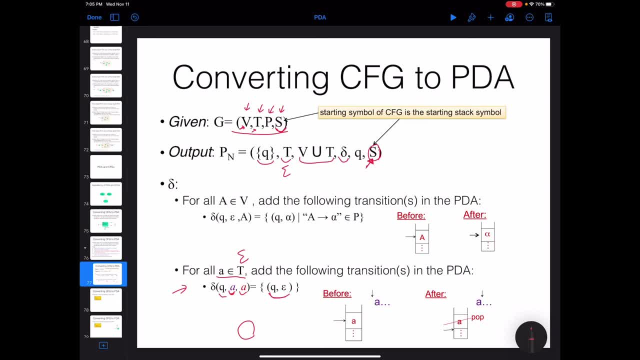 and for all of the variables in our grammar. we are going to add a set of transition that tells me that, okay, without reading anything from the input over the epsilon- um, i'm not going to actually call it epsilon transition, but anyway, we are not consuming anything from the input if the top of 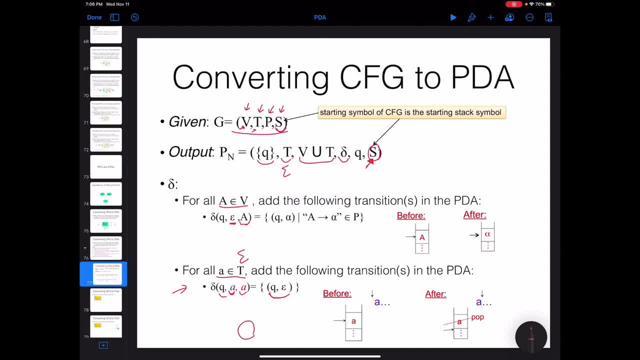 the stack is the variable a. i am going to add one transition for all for each rule that i have in my grammar in this form that, for example, if i have in my grammar something like a, one um, okay, i'm going to have to add one transition, that at state q, without consuming anything from the input, by just seeing. 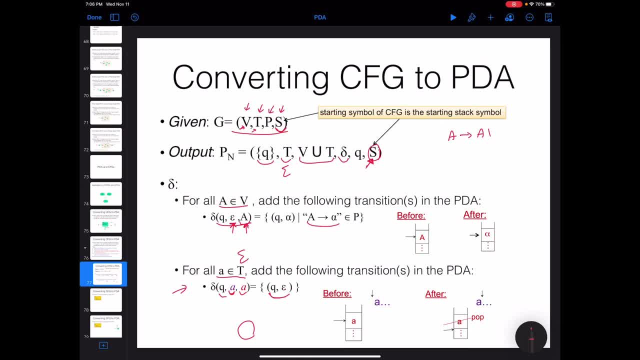 um variable a token a on top of the stack. you um stay at the estate q. you add this transition that you remove, you pop a from the stack and you push the alpha- the right hand side of the rule- so you actually push these two. it doesn't matter how many tokens you have, you pushed all of them. 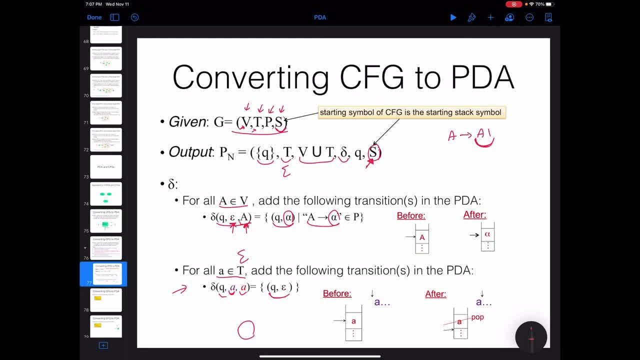 to the stack and from the left to right, so it's not going to be a one-sided transition, but it's going to be a one-sided transition. it means that, um, if you, if you have a situation like this, i don't know what is in the stack except. 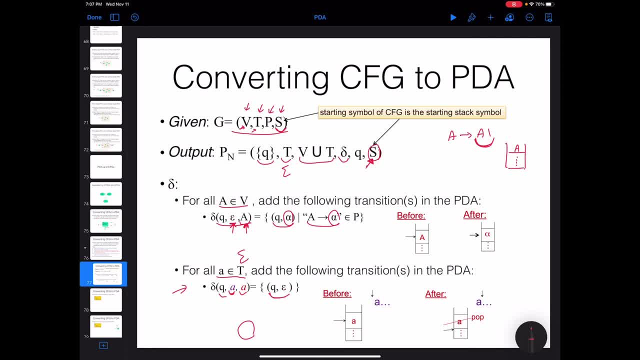 the top of the stack. so if you are going to have a transition like this, what would happen? so that a will be removed from the top of the stack? you push one and then you push a again. so this is just actually the right hand side, okay, um, that's all. this is all of the transition that you need to add. 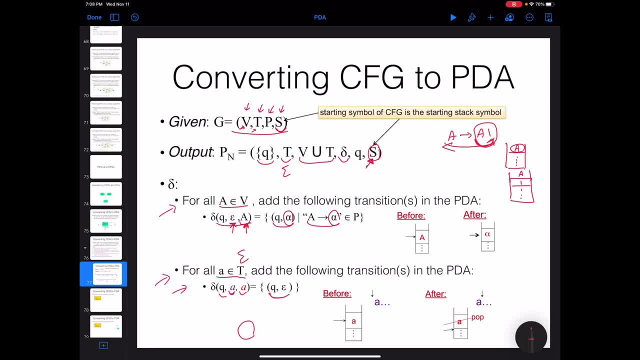 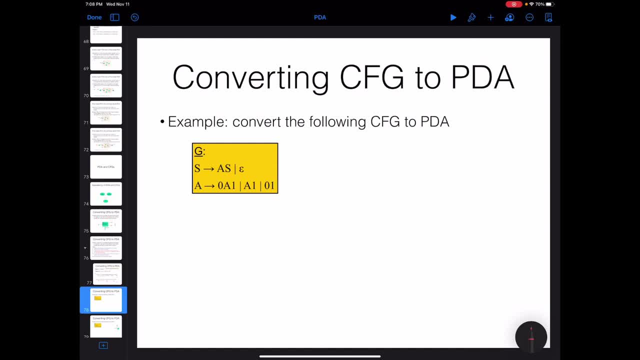 all the transitions for the variables and all the transitions for the terminals. so let me show it to you over um an example here. assume that i have a grammar like this: okay, and i'm going to create a pushdown automata for that. so we are going to have only one estate. let's just call it Q, the starting symbol. 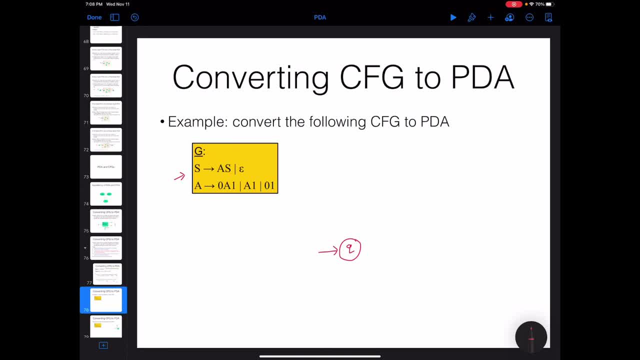 in the. I mean the starting token of the. the initial token of the stack is going to be addressed and I'm going to first add all the transitions for the terminal tokens. the terminal tokens are going to be only 0 and 1 and I'm going to add a transition for each of them. that tells me that. if you have seen, 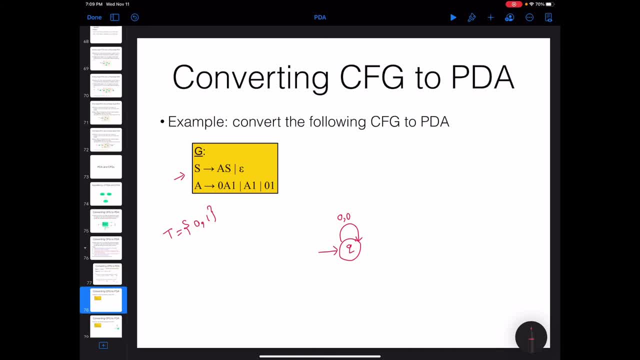 a 0 and the top of the stack is 0 tokens, the ends and the ends and the zero. just remove it from the stack, pop it from the stack. or you, if you have seen one in the input string and the top of the stack is one, just pop it from the stack. okay, now I'm going to add: 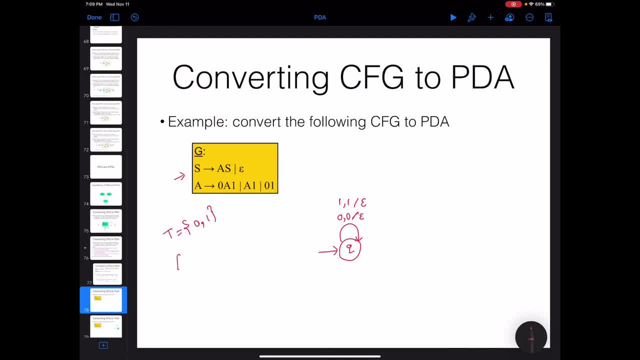 that all the transitions for first for s for s I have to. maybe that's better to start with a. okay, I'll leave it. as for the last one. so I have a variable like a right and it has three rules. okay, for each one I'm going to add a transition. the first rule tells me that 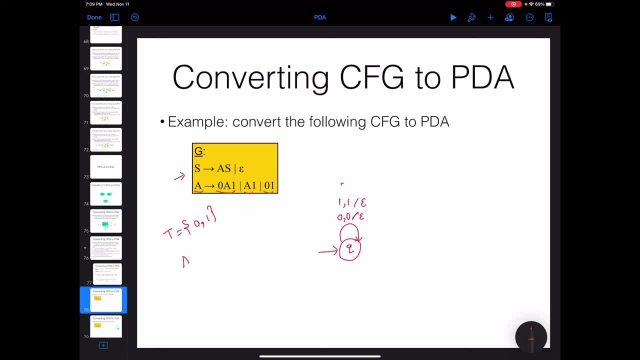 okay, if, without actually consuming anything from the input, if you see the token a on top of the stack, pop it and push um- I mean the right hand side of the rule- to the stack. so it means that one will be first pushed, then a, then zero. okay, so from um you push from right to left so that the left is going the. 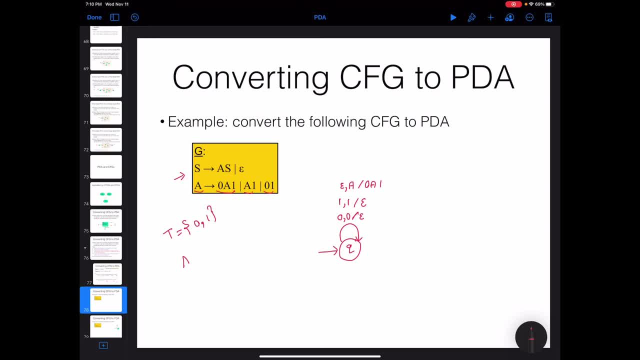 leftmost token is going to be on top of the stack. the other rule that I have is this one. so, again, without consuming anything from the input, if the top of the stack is a, and replace it with one and a, the other transition that I have is the last one, is this one: 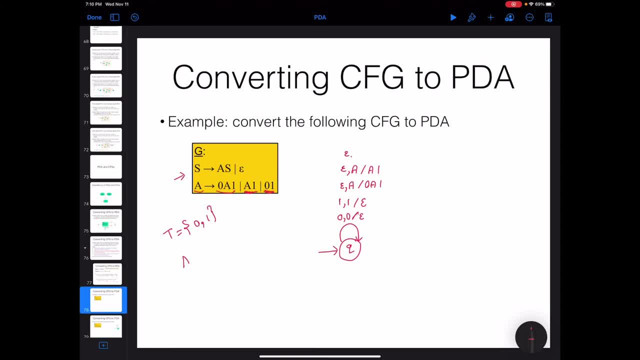 that again without consuming anything from the input. if a is the top of the stack, pop it and replace it with zero one. okay, I'm done with the variable a. the only other variable that remains is s, and it has two um, um, um, um, um, um, um. 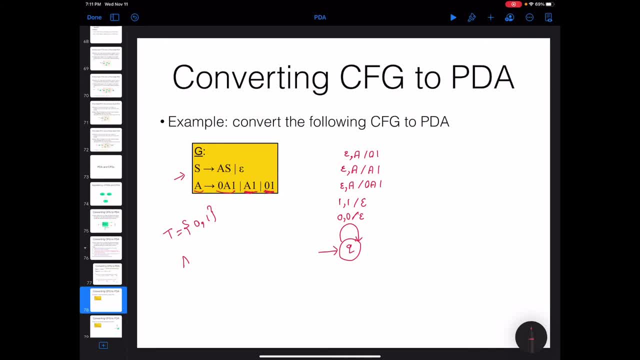 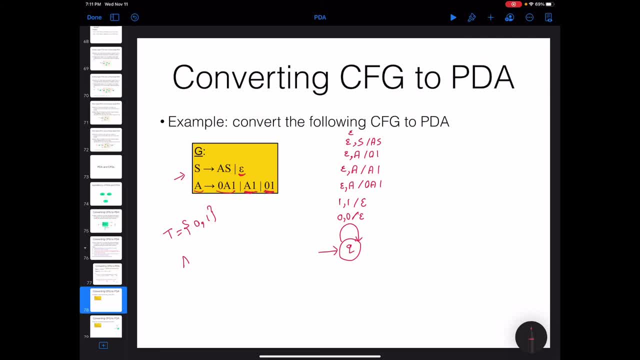 okay, so, without actually consuming anything from the input, if the top of the stack is s, remove it. that's it. this is going to be the pushdown automata. um, uh, corresponding to this grammar here, i am actually showing it to you. uh, over a couple of. 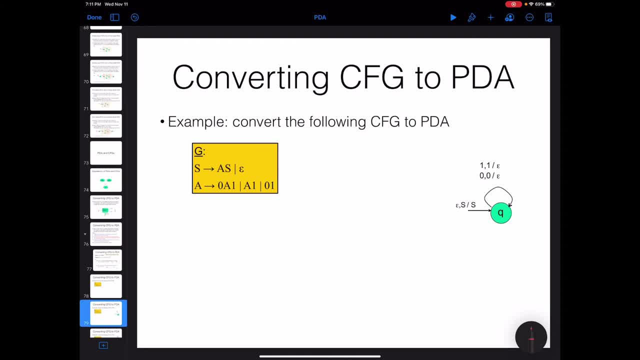 steps, um. you see, always when i'm actually converting to a push non-automata, i'm adding this: um basically just tells that at the very beginning s um has been pushed to the stack. basically s is going to be um, the initial token of the stack. okay, so if you see something like, 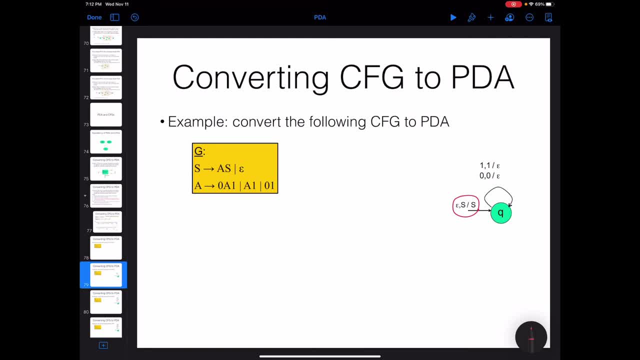 this at the uh, starting state in um, i mean in any source, basically just tells you that whatever you write here is going to be the top of the stack, the initial token of the stack. so all the transitions for a, all the transitions for the terminals and then all the transitions for um, for s. okay, you can see that. 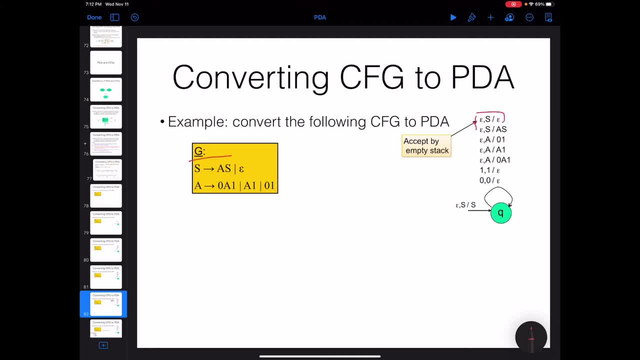 here. we would make sure that, in fact, when by um, i mean this grammar, would make sure that s will be disappeared from uh, your string at some point right, and your push-down automata will remove s from the stack at some point. okay, now let me actually show you how um this push-down automata. 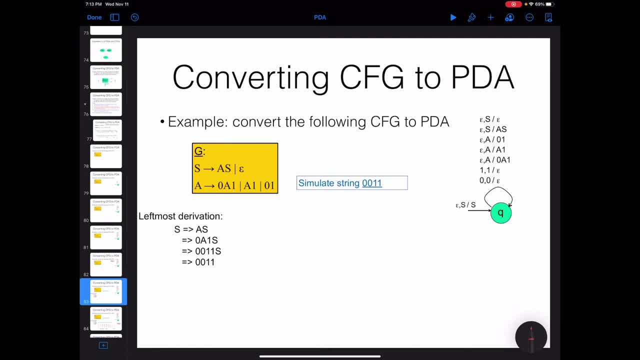 is going to work over s3. basically, what we did by creating this push down automata was um. we basically just try to simulate um, the leftmost derivation for um, each string or on the grammar. okay. so basically these actions that i we have written here helps us to in fact simulates the 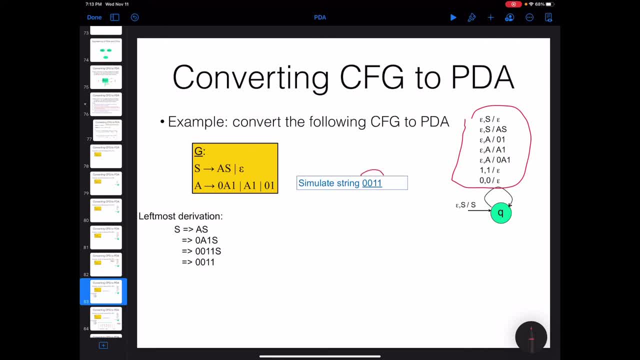 If I have a string like this, generated by this grammar, the leftmost derivation for that is going to be like this: S goes to AS, then A will be replaced with 0A1, and then A will be replaced by 0A1 here, and then S will be actually removed. 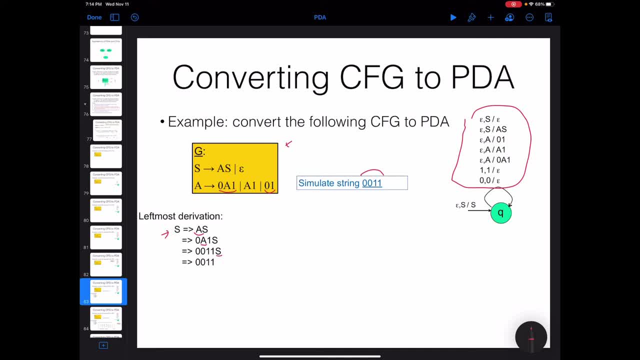 I go to epsilon and remove. So this tells me that how this leftmost derivation tells me how the grammar generates this string. What the push-down automata that we have created does is exactly just simulating what would happen in the leftmost derivation. 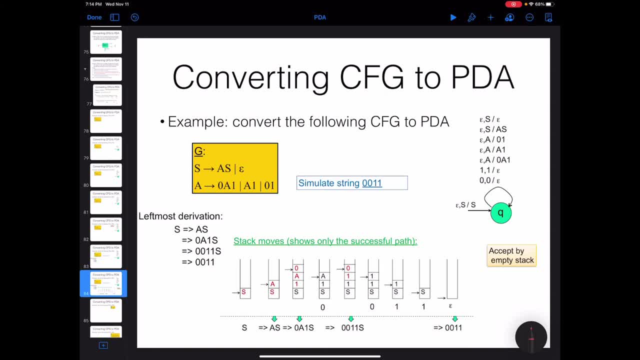 So this is exactly actually showing you this simulation That let us actually just see. Let us see that what we are going to do over this string. You start from this situation: We don't have anything except the initial token of the stack, which is S right. 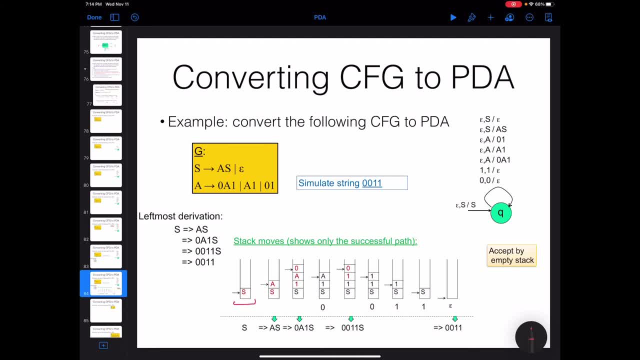 Then so, if you think about all of these actually transitions, the only transition, the only possible transition that we have and is going to actually work, except this one, which removed S, And this is not going to actually generate the. I mean, this is not going to accept the string is this one. You have to use this transition. 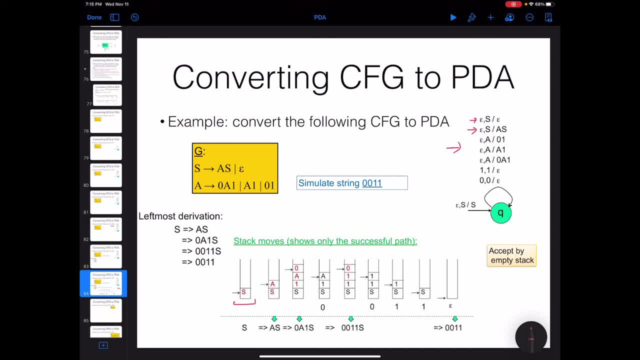 So, over this transition, it tells me that don't consume anything from the input. If the top of the stack is S, replace it with pop it and replace it with AS. So this is going to be the next step. You can see that this is exactly the first step in the leftmost. 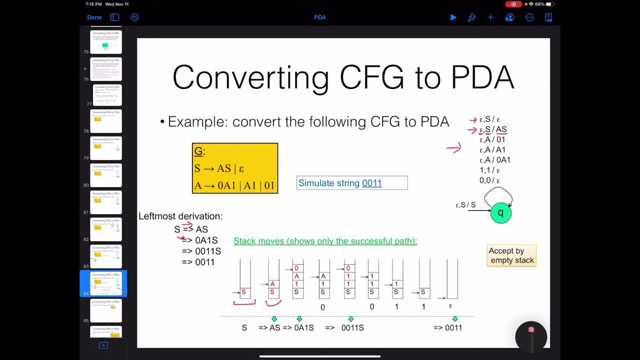 Sorry, This is the first step in the leftmost derivation. right, This is the first step in the leftmost derivation. Then you have A on top of the stack. You can actually go with any of these transition, but the transition that will, at the end, accept this string is going to be this one. 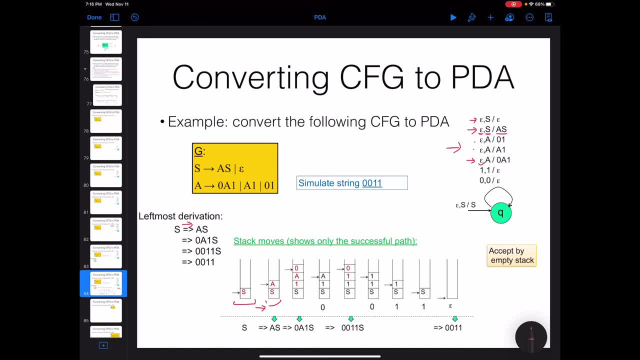 So we don't again consuming anything from the input. This string is still. we haven't actually read the input, this thing we are still actually over working over this transition. The top of the stack is A right. Just pop it and replace it with 0, A1. 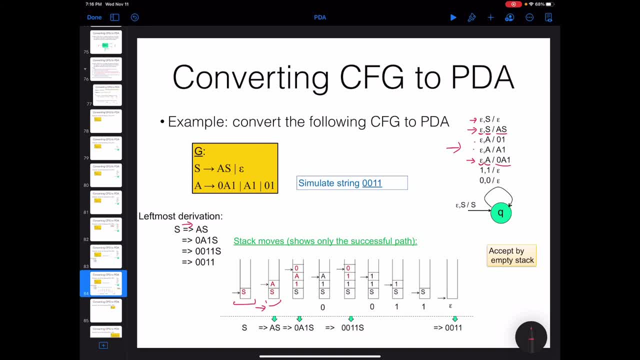 So what would happen is that A will be popped from the stack and 1, then A, then 0 will be pushed to the stack. Okay, So basically this is exactly the same, The second step of the leftmost derivation. then you would: um, actually the top of the stack is 0. 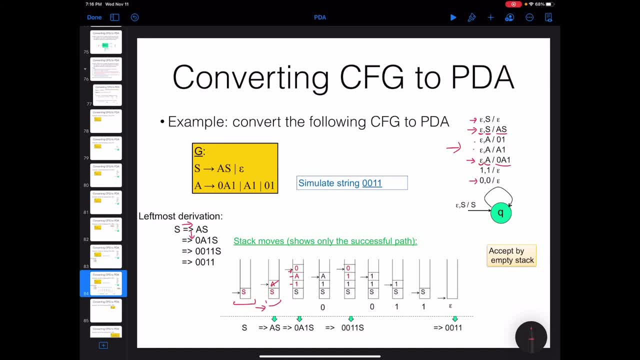 The only transition which is possible for you is this one, which, basically, is telling you that, okay, the first token of the input string has been generated, and it's just like you have read this one and you are here. No, the first token has been. 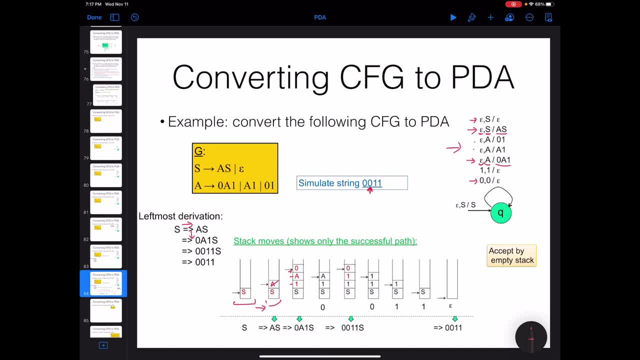 Consumed. Okay, The next step is that- okay, I have read. the top of the stack again is A, so I should use one of these transitions. right, I can use any of them because none of them is using any input string, but the one that will end up to accepting the string is going to be this one. 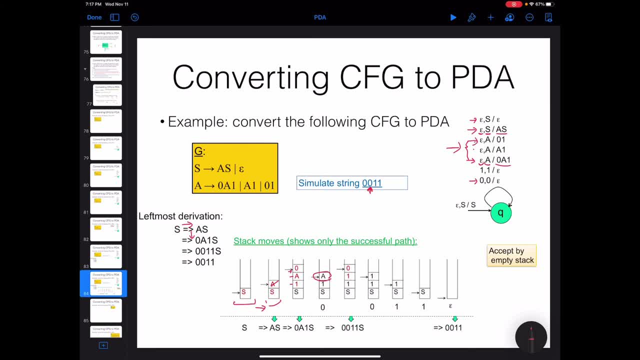 So let's actually just um apply that transition. If I apply that transition, It A will be removed from the top of the stack and 0, 1 will be pushed to the stack, and I'm not going to consume anything from the input. 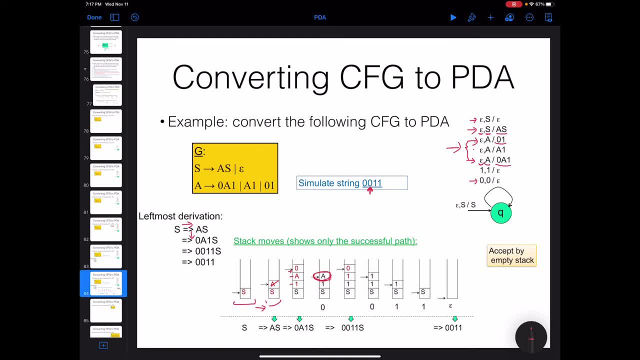 Still, I'm going to be here. So 0,, 1 and 0 will be pushed to the top of the stack. You can see that this is exactly the next step in the um leftmost um derivation right. 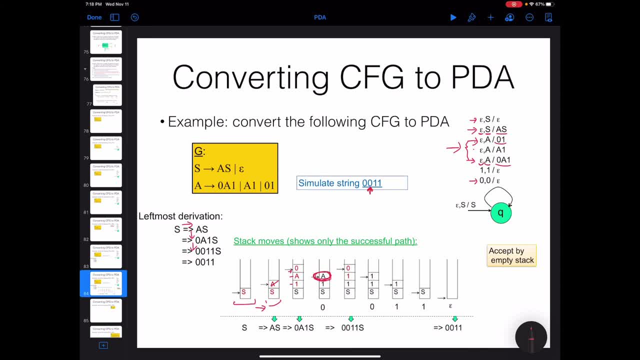 We re. we removed A and replace it. We replaced it with A, Um 0, 1, one of the actually rules. here I mean the step that we have done in the leftmost derivation, then in the next step, the top of the stack is 0. 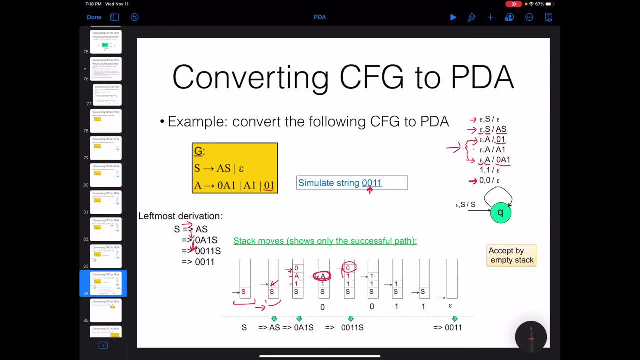 Okay, The only transition which is possible is this one: You have um 0 on top of the stack and you have 0, um as the next token, So you will consume it. Um, so you will remove it. 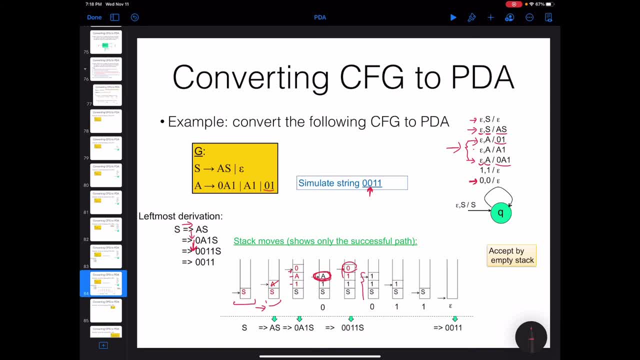 You will remove it from the top of the stack and you reach to this situation. So the next input is token is going to be one. The top of the stack is one. The next input token is one. So I have to use this transition. 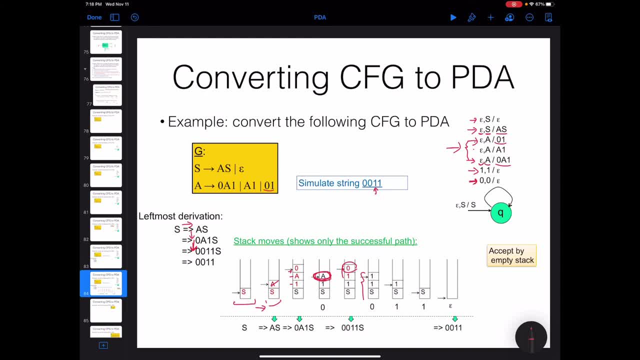 You just match them and you remove it from the stack. Um, um, the next token in the input string is one. The top of the stack is one right. The only transition is possible is this one: You just pop it. pop one from the stack. 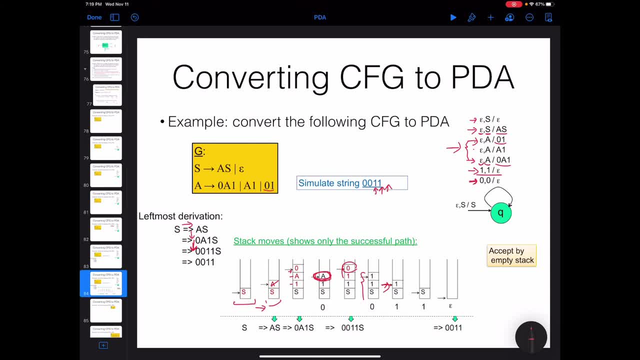 Then you are done with the input string. What would happen to the stack? In the stack you only have S. okay, You can remove it from the using this transition. you can remove it And your stack will be empty, which basically means that you accept this string. 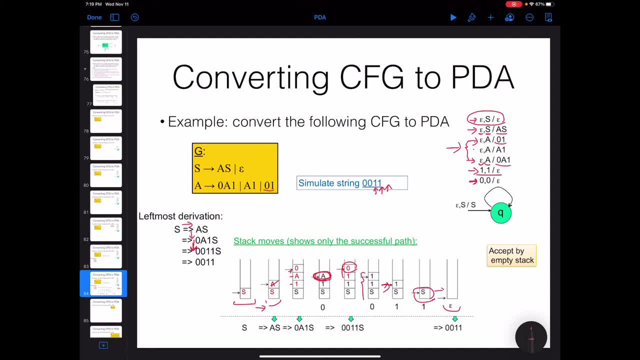 And this last action that you have is exactly the last step of your um leftmost derivation. when you will be um, you are generating this string. So basically, the pushdown automata, basically I have, I'm using basically a lot. 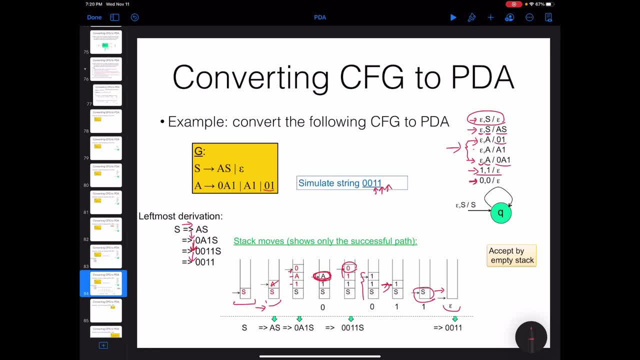 Okay, Pushdown automata just simulate what we did in the leftmost derivation, Um, to generate any string. So, whatever is your grammar, um how we generate a string, the pushdown automata just simulate that to accept the strings. 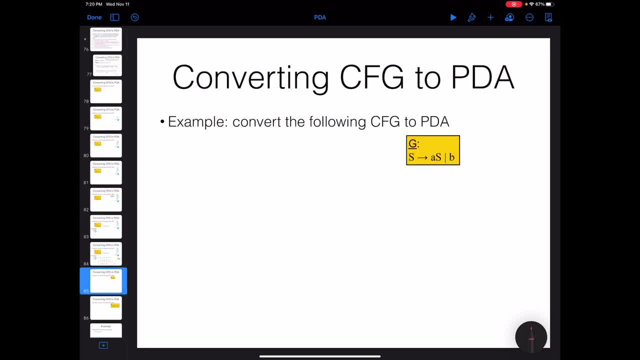 So let's see another example. I'm going to convert this context free grammar to a pushdown automata. again, we are going to have only one state. let's just call it q, whatever, and the s is going to be the initial token of the stack. we have the set of terminals or the input strings. input tokens are going to be a. 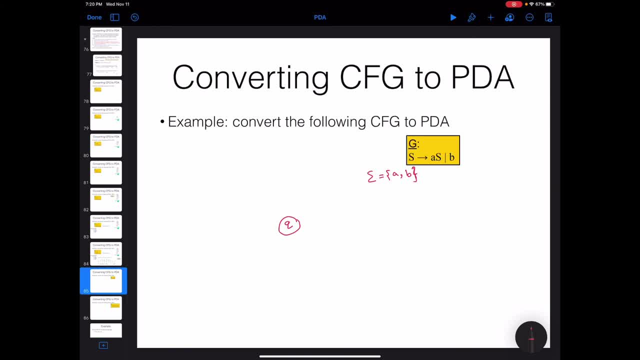 and b. i'm going to add one transition for each one. so if the top of the stack, if the input string input token is a and the top of the stack is a, just pop it. or if the input is token, the next input token is b and the top of the stack is b, just pop it, and we only have one variable. 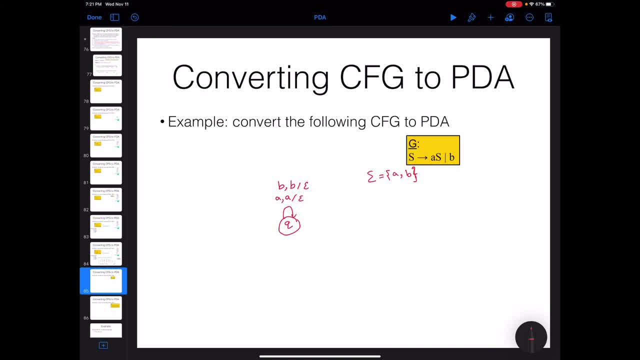 but we have two rules for that. so it tells me that if the top, if we don't actually consuming anything from the input, if the top of the stack is s, you can pop it and replace it with push a, b to the stack or without consuming anything from the stack. 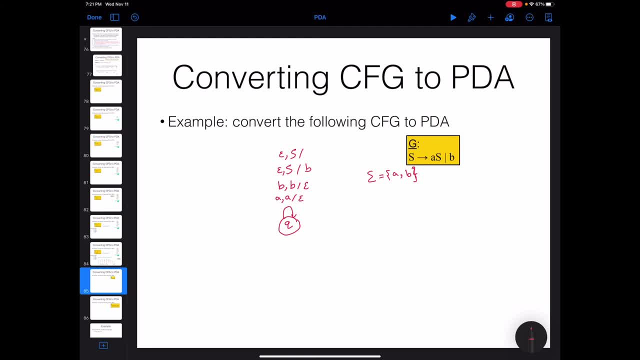 you can. if the top of the stack is s, you can push s and a to the stack, and that's it. this is going to be the pushdown automata for this. let's see another example. remember this grammar. this grammar was generating arithmetic expressions with a very limited form of the identifiers. 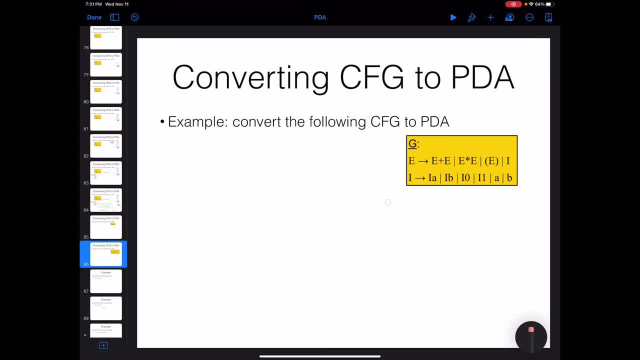 so here the set of terminals or input alphabet is going to be a, b, 0, 1 plus star, open parenthesis and close parenthesis. okay, all of these are going to be the terminal tokens in the grammar right, so all of them are going to be a part of the 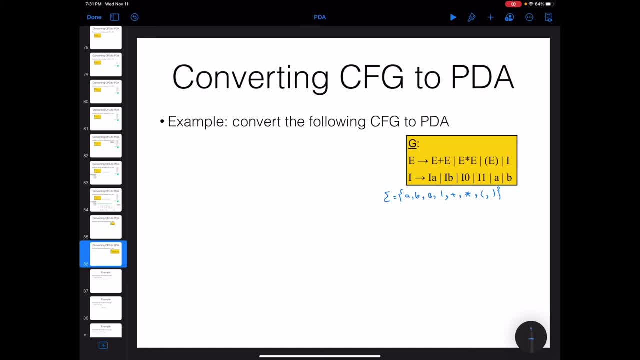 input, the valid input tokens. so when you are, we are creating the or input or pushdown automata, we are going to have one, only one state and you first add all the transition for all of the tokens, for all of the terminal tokens. so if you see a and the top, 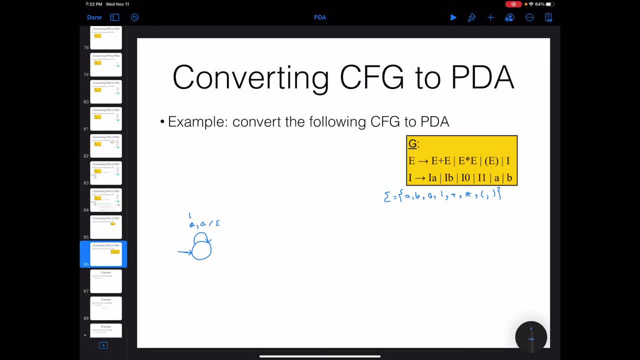 of the stack is a, pop it. if you see b in the input and the top of the stack is b, pop it. if you see zero and the top of the stack is zero, pop it. if you see one and the top of the stack is one, pop it. 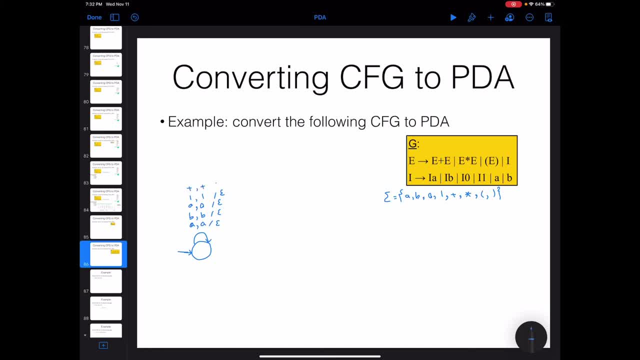 if you see plus and the top of the stack is plus, pop it. if you see a star and the top of the stack is a star, you pop it. if you see open parenthesis- the top of the stack is open parenthesis- pop it. if you see close parenthesis, they don't really. 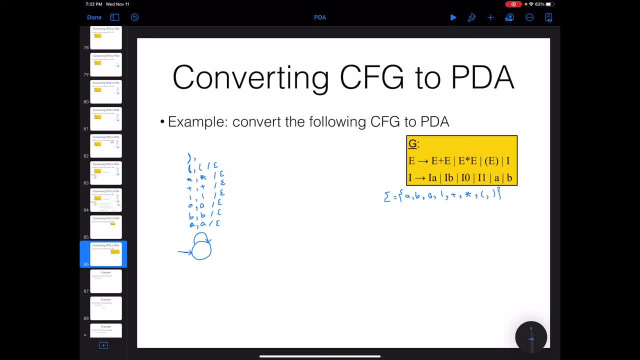 look like open and close parenthesis, but anyway, you please excuse my handwriting. okay, we have covered all the terminals. i don't have a space, so i'm going to write the rest of the transitions here. so now i'm going to write the transitions for the variables first, for i 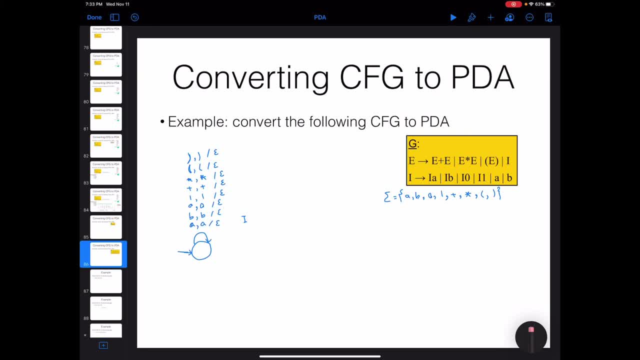 so now i'm going to write the rest of the transitions for the variables first, for if you, actually, without consuming anything from the input, if the top of the stack is i, you replace it with a and i. so i'm reading it from the right to left to actually tell you that. 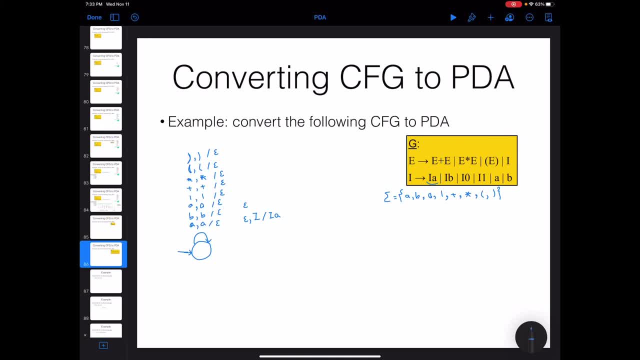 i is going to be the top, without consuming anything from the input. if the top of the stack is i, you can. if you, actually, without consuming anything from the input. if the top of the stack is i, you can pop it and replace it with b and i, you can replace it with. 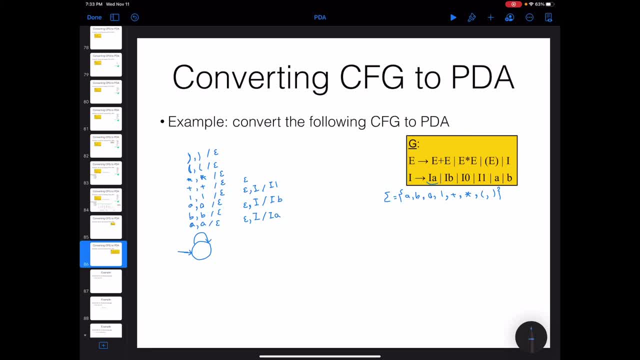 one and i. you can replace it with zero and i. you can replace it with a. you can replace it with b. so these are all the transition for i. i need to add all the transitions for e as well, so, without consuming anything from the input, if the top of the stack is e, you can replace it with 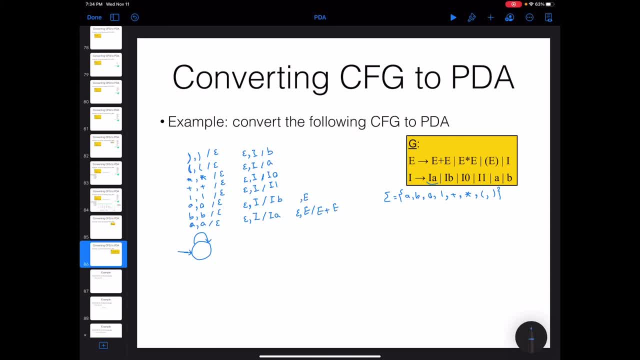 e plus e, or you can replace it with e multiply by e, or you can replace it with e with open parenthesis, e close parenthesis, or you can replace it with i. so now we have created the transitions for all the rules, all the terminals. um, we are done. this is going to be the pushdown automata. 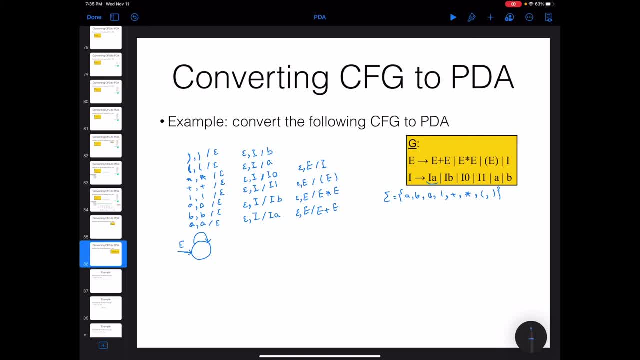 and the starting symbol. be careful: the starting symbol is going to be e. just to make sure that it is clear, the starting symbol is going to be: you can basically try to, for example, generate a steering using this grammar, something like it's as simple as a plus b, for example. 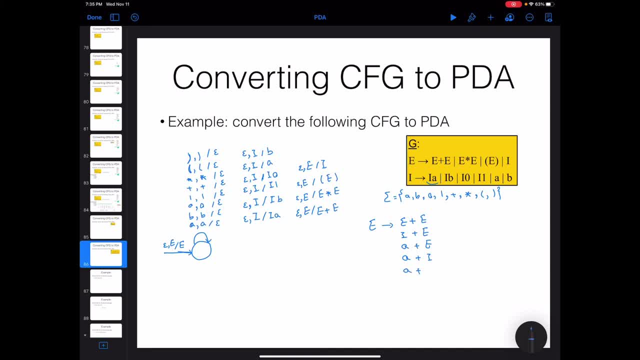 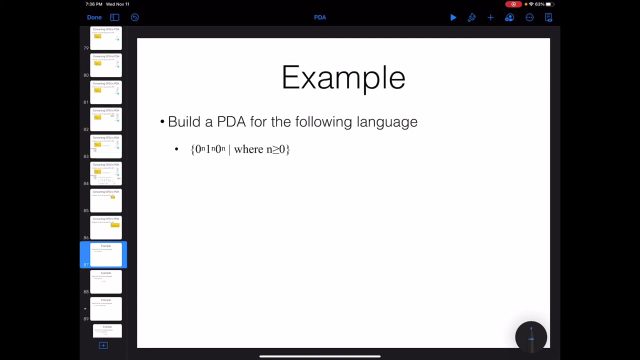 this is the leftmost derivation: right to generate a plus b. just try to see that. what, uh, how the um? this pushdown automata is going to accept the string a plus b. that just actually helps you to digest it better. so let's see another example: um. create a pushdown automata for this grammar. 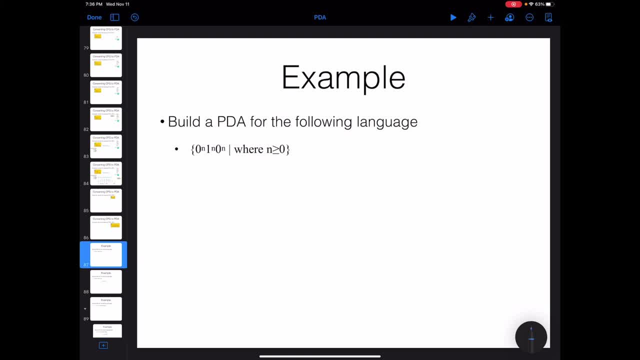 is it possible? can we create a pushdown automata for this grammar? unfortunately not. this grammar is not context free language and we cannot create a pushdown automata for that. i mean no, it became more clear for you that why. um i mean a grammar um. a language like this is not a context free um language. 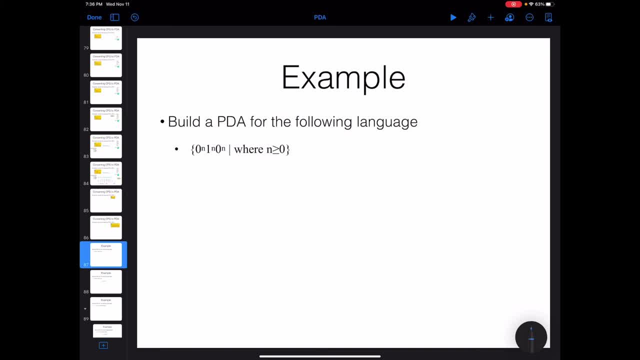 um, if you think about your machine, just think in this way that you can read your string from left to right only once and you have access to a stack. can you recognize the strings? which belongs to this language or no? you can see that for the number of zeros this language force you to have. 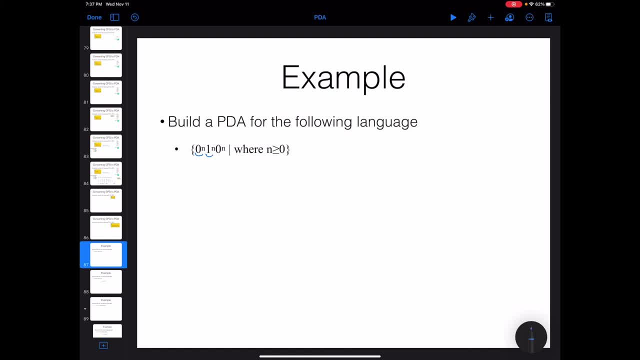 n number of 0s, followed by n number of 1, followed by, exactly again, n number of zeros, to count and make sure that the number of 0s and the number of ones are equal. you can use a stack, right, remember we actually, for each 0 that you read, you can push it to the stack and 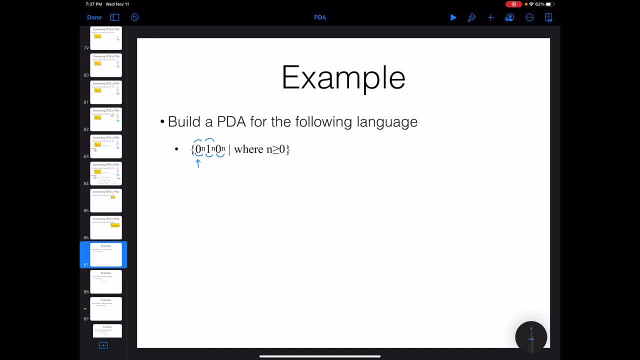 keep a token in the in the stack, then, for to make sure that the number of ones is equal to the number of zeros, you can pop those from the stack. pop those, all of the tokens. but the thing is, when you are you reach to this point, you don't have any other indicator to count the number of. 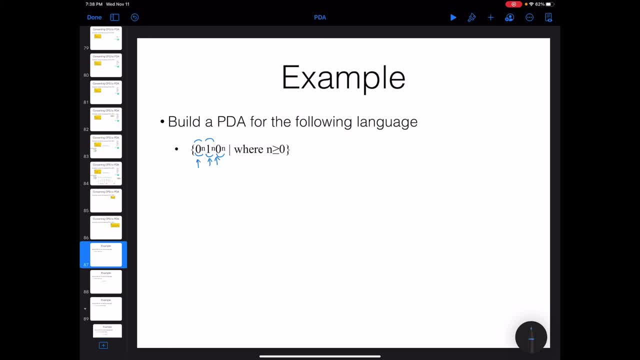 zeros remaining zeros at the end, and make sure that they are going to be equal to the number of zeros and ones that you have seen before. the stack is empty and i don't know how many zeros or ones i have read so far. so now it is clear that, yes, the pushdown automata, a machine that reads. 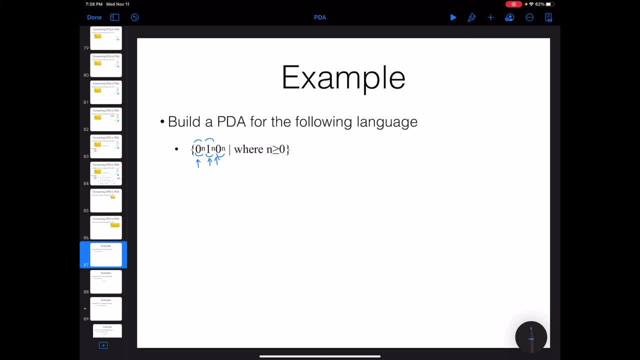 the strings from left to right and only have access to a stack, cannot accept, cannot actually represent this language. this is not a context free language. how about this one? all the strings that you know the length of them are even and the string has been repeated. okay, something like one, one or, for example, zero one, zero one. can we create a pushdown automata for? 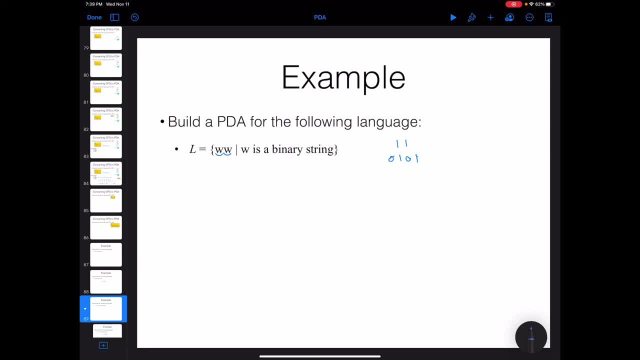 this language. we know that we can create a push down automata for this language that whatever is the string W, reverse it at the end. this is a poly compr, this is a poly algorithm with even lengths. right. basically, we can do it because we have access to um, a stack, whatever is. 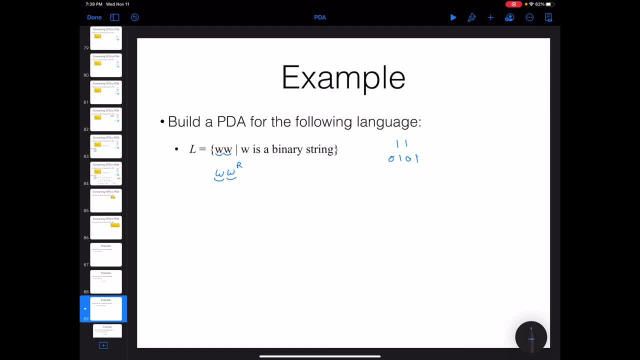 whatever is um the string W, you can push it to this like: and your stack is going to be the first in last out or last in first out. type of structure: data structure- right, so the last token that you have read from w, you can match it as the first token of the reverse of w, so it is possible to. 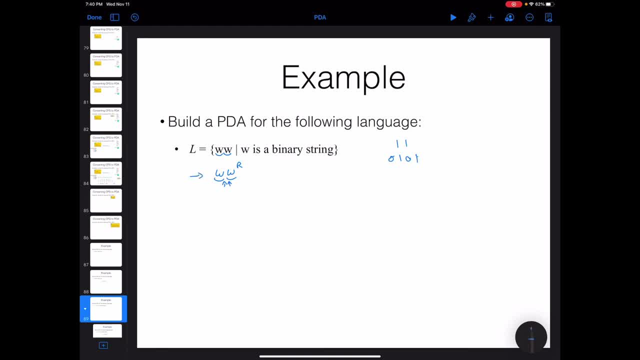 create a pushdown automata for this string, but how about these type of strings, can we? no, we can't, because whatever is going to be actually at the middle point, whatever is the inside w, you should actually just read it as the from the bottom of the. 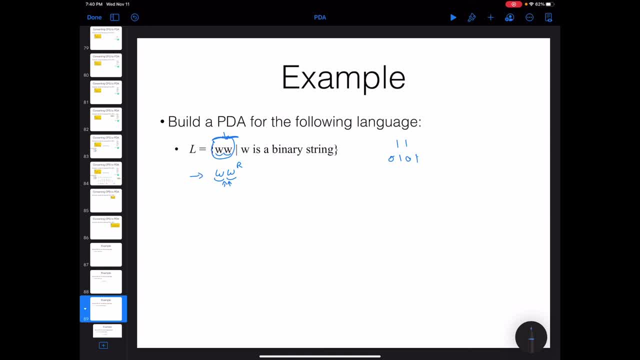 you know a stack and you don't have access to it. you only have access to the top of the stack. so this type of this language is not going to be context-free language as well, because we can't not create a pushdown automata to accept it. let's see another example. how about this language, is it? 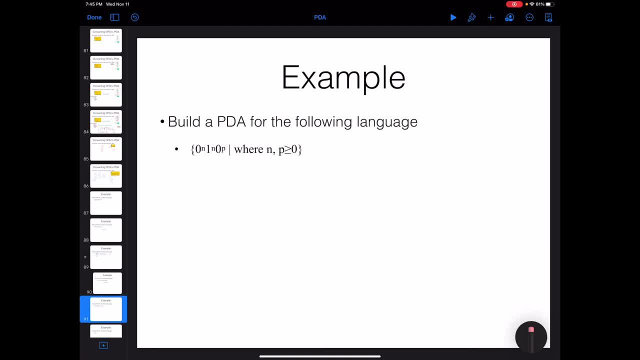 a context-free language. yes, this is a context-free language. this is very similar to this example that we have seen here, but the difference is that we don't restrict the number of zeros at the end to be equal to the number of zeros and ones at the beginning. so this is going to be a context-free. 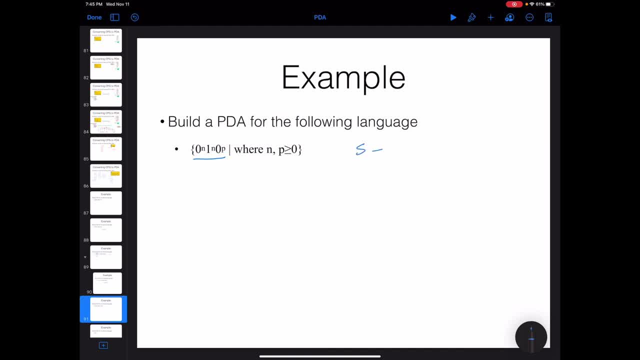 language. we can create a grammar for that something like goes to: a- B. a is responsible to generate the the first part. zero a, one or epsilon, and B is responsible to generate the last part between the first part. zero a, one and b is responsible to generate the last part between 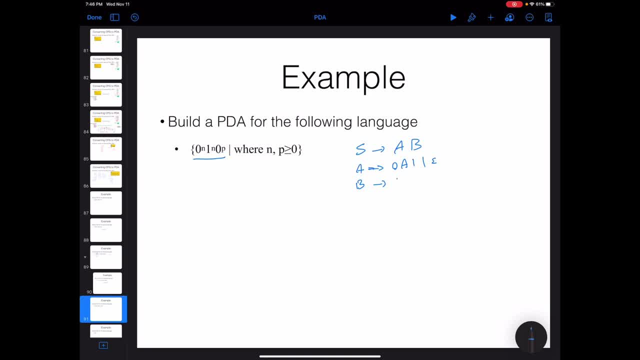 is going to be b, zero or epsilon, okay, this is the context-free grammar for that and we can create a push-down automata for that. i mean, um, i don't want to actually go through that as the, i mean the theorem and that proof that convert the context-free grammar to push-down automata. 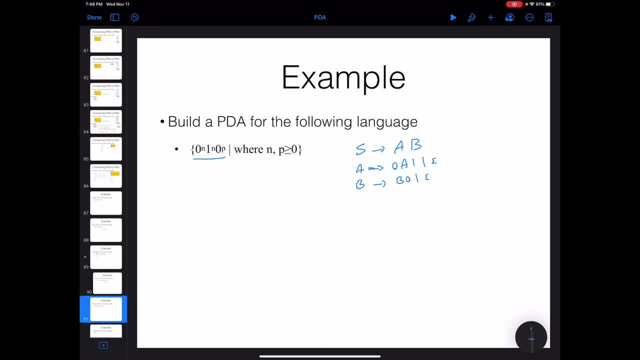 um, just forget about that- how we can create a push-down automata for this language. we can think about it as this way that this is very similar to the. you know, the first, very first example that we have seen. just have a state to push all the zeros. 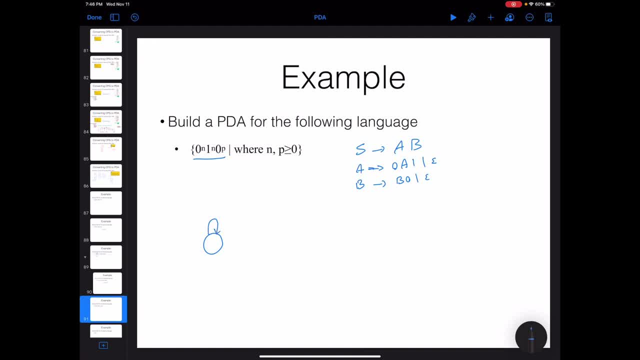 okay, for each zero that. you see, it doesn't matter what is the top of the stack. okay, just consider it as z zero, just push. um, let's just use zero. that makes it actually easier to work on later. for each zero, i'm going to push a zero to the stack and 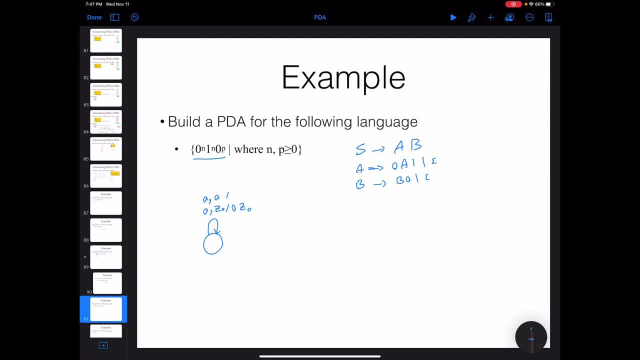 um, if the top of the stack is zero, just push a zero to the stack. and if the top of the stack is the stack, um, without consuming anything, i'm actually creating a non-deterministic push-down automata. for this one, you can create a push-down um deterministic push-down automata. 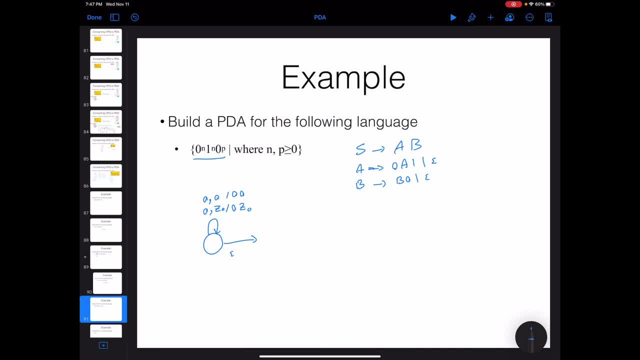 um, as well, but um, just to make it easier, i'm creating a non-deterministic one. so if it is z zero, um, just keep z zero and move to this state. this state is going to just pop the ones. or if the top of the stack is zero, just don't touch it and move to this state. this: 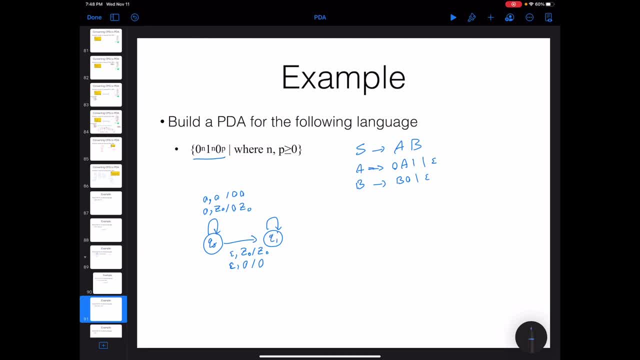 state: let's just call this one q0, q1, q1 is popping the all the ones that you have pushed, so that's going to be one, and the top of the stack is zero, pop it. um, only pop if the top of the stack is zero. 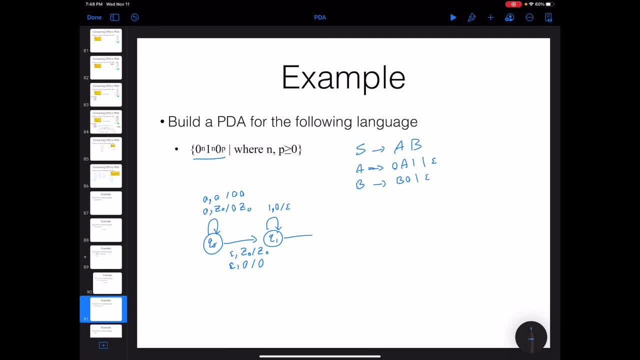 or you can move. so it's just like we have pushed all the zeros, all the beginning zeros, to the stack in the q0 and then in q1 we have popped all the zeros corresponding to the ones that we are reading and then we can move it. 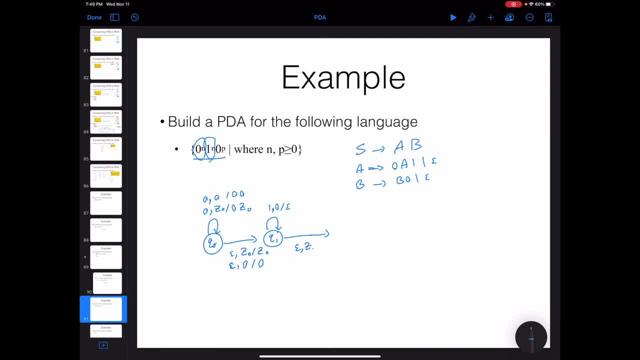 if we have read all of the zeros and ones and they are all matched, you can move to this state q, temperature three, which is an accepting state, and for all the zeros that you see, if the you see a zero and the top of the stack is z, zero, and 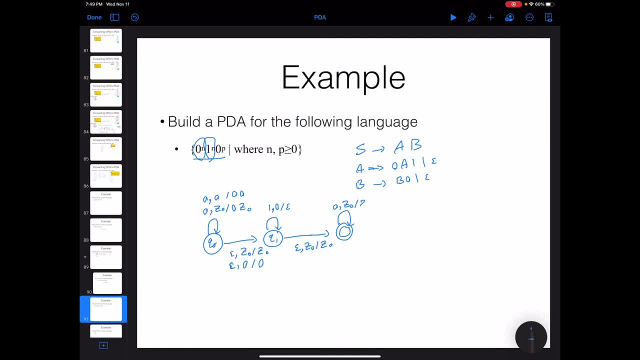 um, just keep. keep z zero here, okay, so this is going to be the only um possible transition, so you can read as many number of zeros as you want here and stay at the final state. so this is a pushdown automata that accepts y final state. i just designed it in this way because i wanted 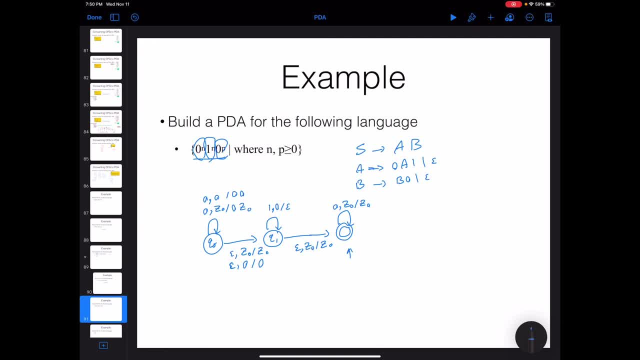 to actually give you the the idea of how to think about the um, an algorithm for your pushdown automata, not just converting the grammar to a pushdown automata that accept y final state. how about this one? can we create a pushdown automata for this?